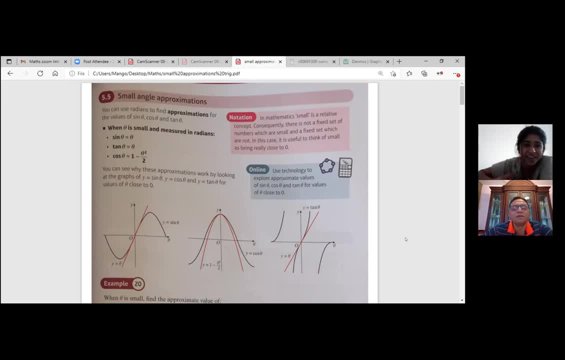 So I'm guessing you just have to know that. Have they shown that? Why is it so? I mean, yes, you could start from here, But did they ever explain? you like in the book? Because this seems to be the beginning of this chapter. 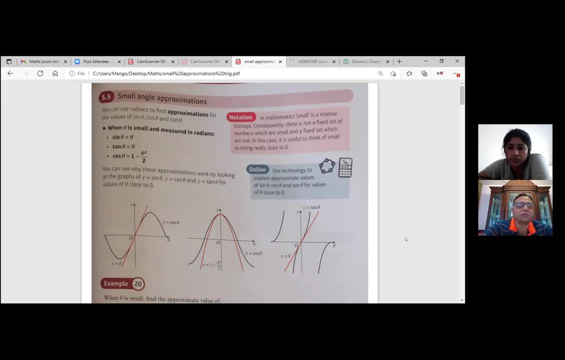 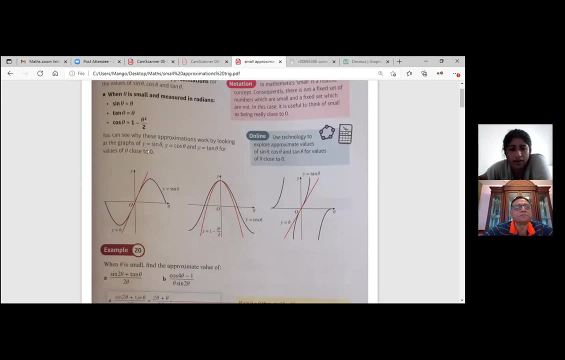 Yeah, it is. Have they explained you why it is so? I think there's something about the graph. Can you please read the next paragraph also? Yeah, so you can see why these approximations work by looking at the graphs of: y equals sine theta, y equals cos theta and y equals tan theta for values of theta which is close to zero. 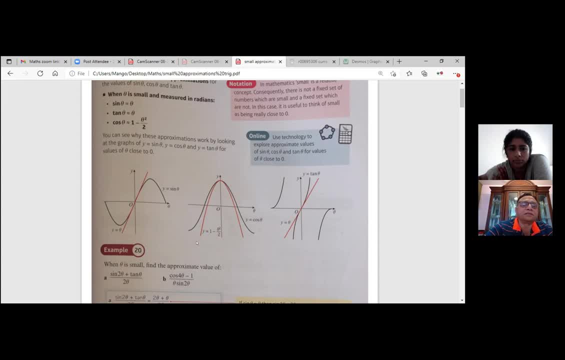 So close to zero really means that you are at this origin. Let me just mark these points for you, right? So at this area, right, This is this area which you're talking about. And for tan, it is this area which you're talking about. 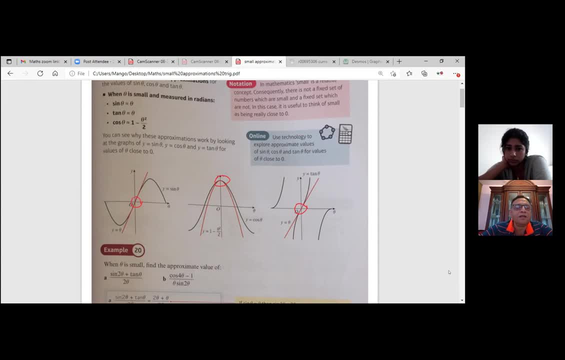 Yeah, So when you are very close to zero, then you see that the line y equals to theta which is written here- y equals to theta matches with y equals to sine theta. That's what they're trying to say, correct? 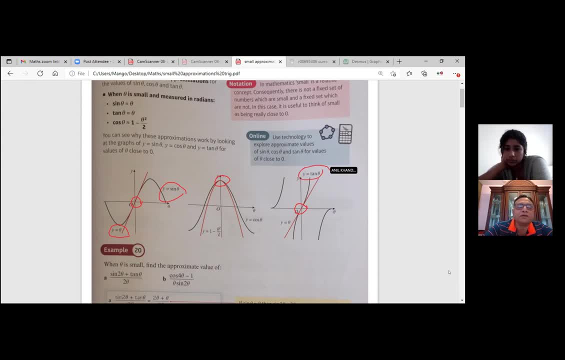 Yeah, And for tan theta also. you can see, this is kind of difficult to realize, but one minus theta, squared the curve, is given to you. It's a parabola, right Yeah, Which is opening downwards kind of thing. You can see this parabola. 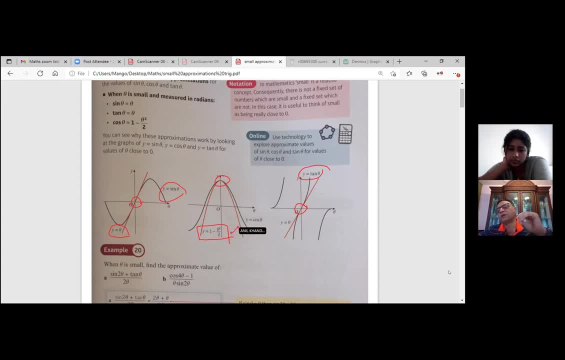 Yeah, Yeah, Yeah, Yeah Yeah. On the top it is equal to almost one, correct? So we know cos zero is one for sure. but close to cos zero means approaching that value. It is approaching to the radian value, the equivalent one minus theta squared by two, by this formula: 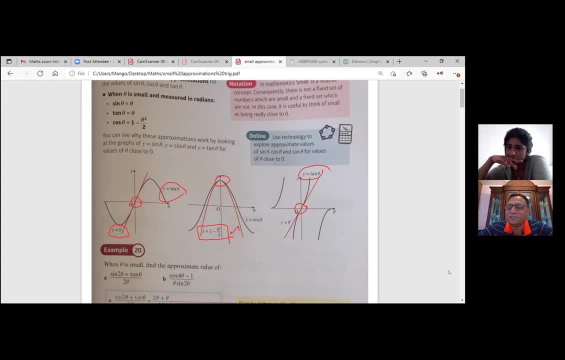 Okay, So actually you had shared with me what difficulties you are facing. I just wanted to have a look at what you, what is there in your book. but I think I'll begin from you know, introducing you to this formula. 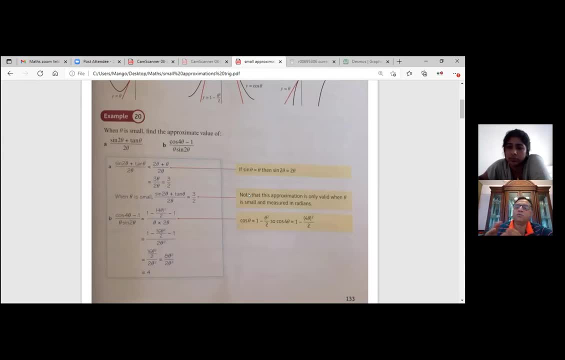 Okay, Okay, Yes, Yes, Okay, Okay, Yes, Okay, Okay, Okay, Okay, Okay, Correct Okay, Yes, Correct, Yes, Yeah, Okay Okay, All right then, Okay, Correct, Correct Okay. 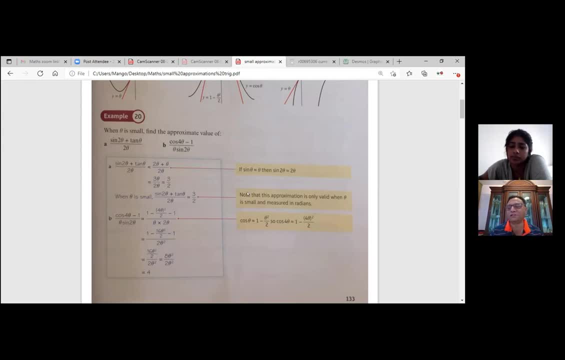 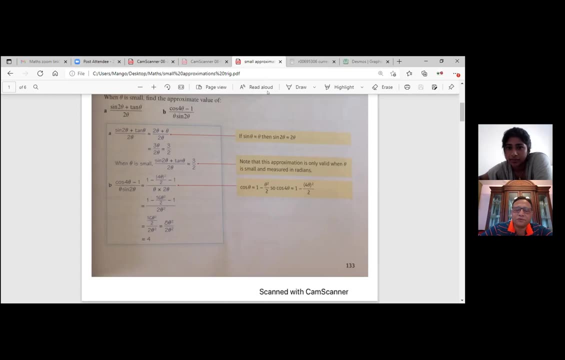 All right then, Okay, Okay, Let's see. Okay, Okay, Okay, Yeah, I think we're finished Theta very, very close to zero. Is that clear to you, Right? Yeah, yeah, So, yeah, So I have my lesson for you. 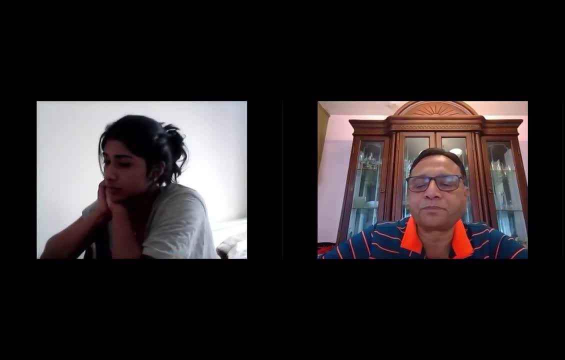 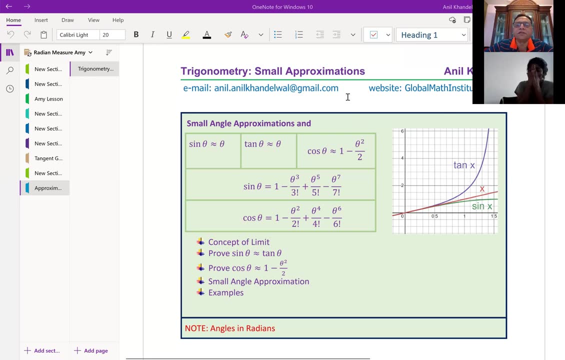 We'll just work on that, So let me just share the screen. Okay, So my approach will be slightly different from what we have seen here, But to begin with, I have the same things that you showed me, which is we're talking. 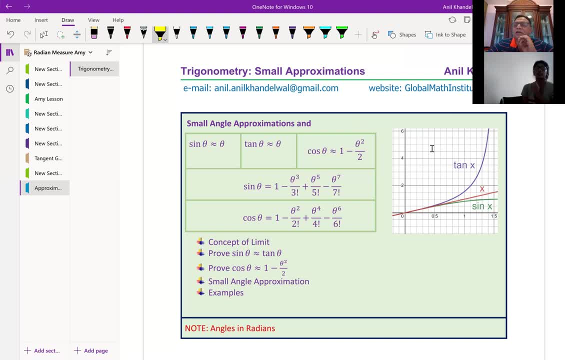 about small angle approximations, correct. So when the angle is very, very small, then sine theta approximates to theta, tan theta approximates to theta and cos theta approximates to 1 minus theta squared over 2.. And always remember we're talking about the angles in radians, right? 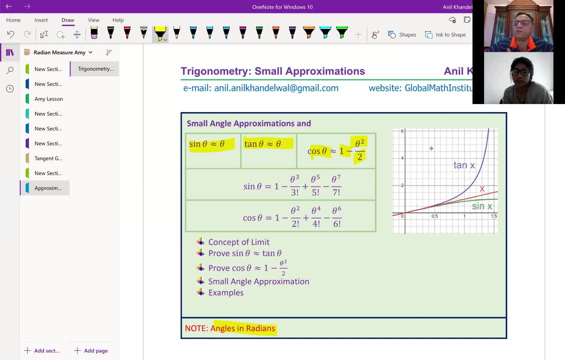 Not in degrees. Radians is a default unit and we are working with angles in radians. Is that clear to you, right? Yes, yeah, Some more equations which we have not dealt with so far are written here. I'm writing a value of cos theta. 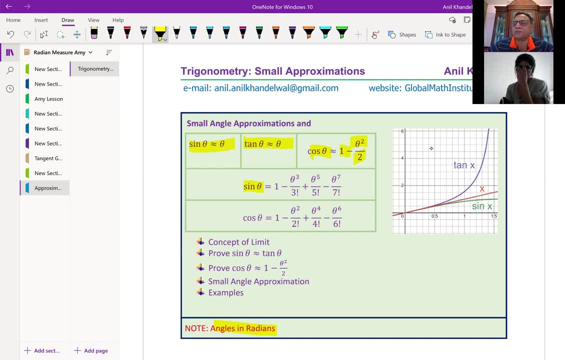 It could be written as a series. You know that's sine theta and cos theta. You can make a note of this series. Sine theta is equal to 1 minus theta cubed over theta 3 factorial. When I say 3 factorial it means 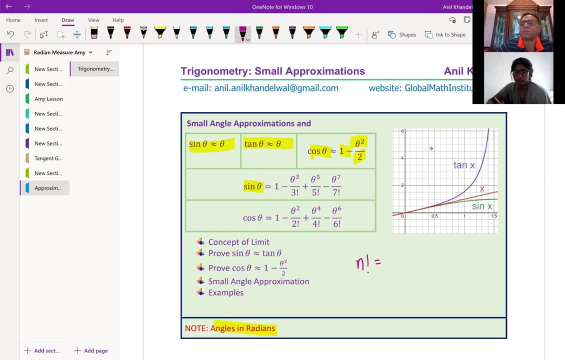 Let me write what n factorial is right. So n? factorial is basically product of numbers till n, right. So you can say: 1 times 2 times, 3 times, 4 times, right till n, is that okay, Yeah? 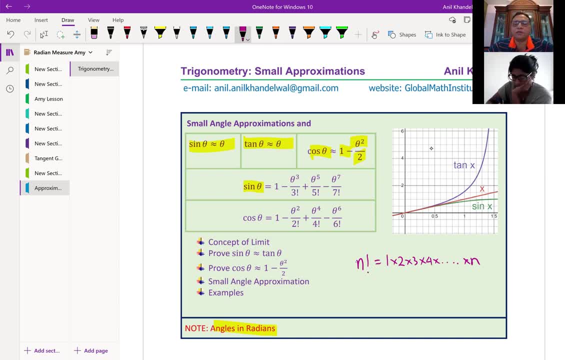 So product of n numbers 1 to n is n factorial. So when I write 3 factorial, 3 factorial really means 1.. I could write also decimal here. That is not a decimal, but a sign for product right. 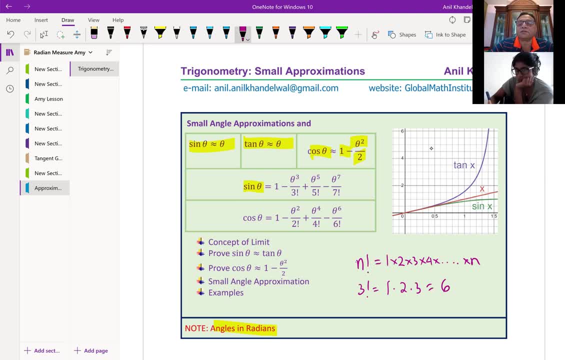 1 times 2 times 3, which basically is 6, right? So that is what 3 factorial is 2 factorial. if I write it is 1 times 2,, which is 2.. And if I write what 5 factorial, for example, 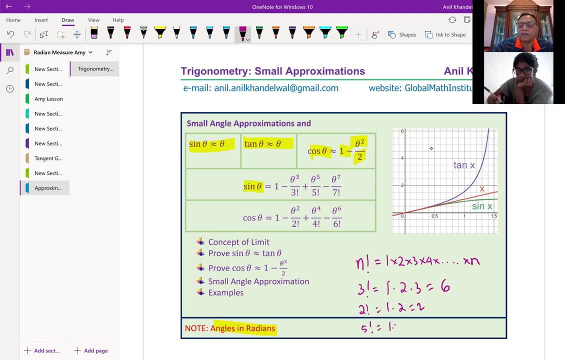 then it could be written as: 1 times, 2 times 3 times, 4 times 5, correct. And 4 times 5 is 20.. 20 times 6 is 120, right. So that is the convention. So sine theta is 1 minus theta cubed over 3 factorial. 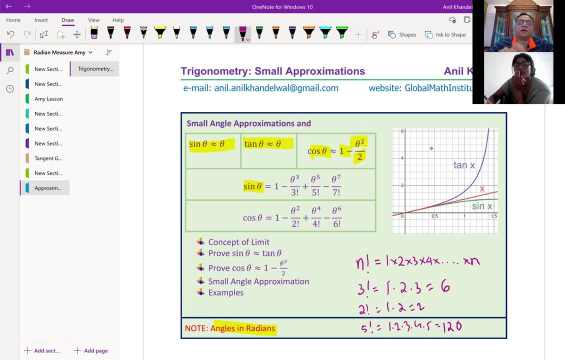 plus theta to the power of 5 over 5 factorial. Similarly, cos theta has a value of 1 minus theta squared over 2 factorial. So these are the series which gives you approximate value of sine theta and cos theta right. 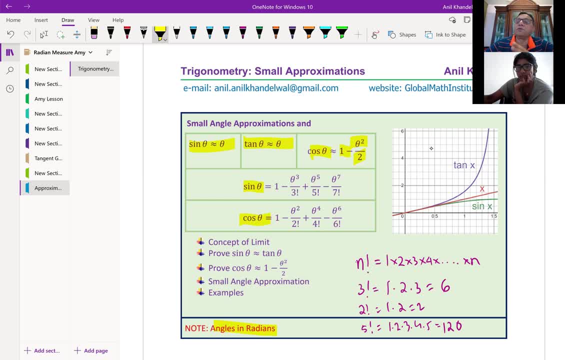 You're talking about approximate values. We will look into the binomial expansion and the special usage of binomial expansion to get the values of sine theta and cos theta. That will be a different chapter. However, this will be dealt with in that chapter. 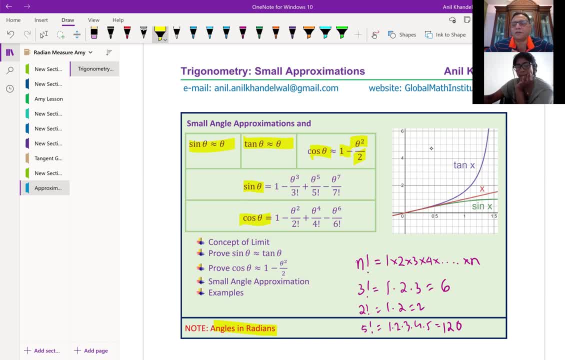 Is that clear to you? It's also part of your curriculum and that's why I'm just giving you here. Okay, Now, as I was saying, we'll actually give you a little bit of time, We'll get into the concept of limit, because the thing is: 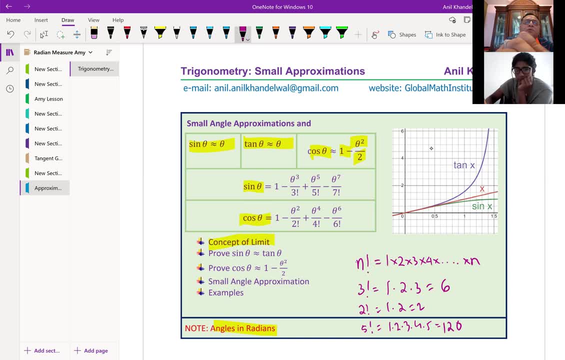 when we say small angles, what does this small angle really mean? When we say small angle, that means what? Well, I could say. well, theta is approaching zero. You get the idea. Small means very close to zero. Is it clear to you? 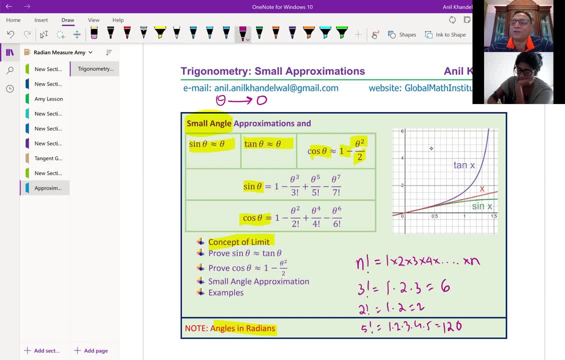 Very close to zero. You'll be surprised, however, that the value for cosine, the theta, could be pretty low. It could be large also. We'll give you a value which is close to 1%. Zero, Yeah, close to. 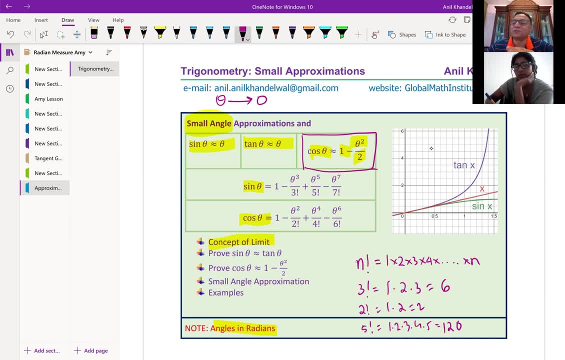 No, no, not theta approaching zero. Even theta equals to In degrees. if I say This is in radius, This theta is in radius, But in degrees, almost about 30 degrees also, if you choose this radian value. 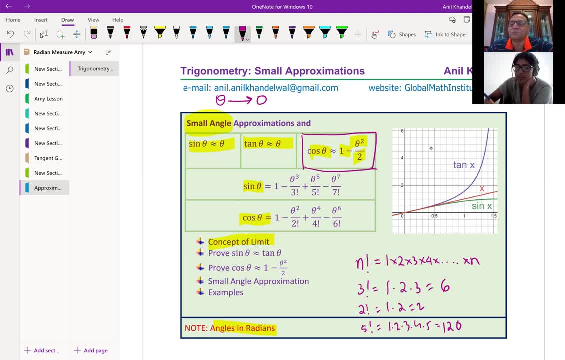 it will be pretty close, within 1% error. Oh, We'll learn that. So it is not just approximations: a very accurate approximation, many times used for many, many results And, when we're saying theta, very close to zero. 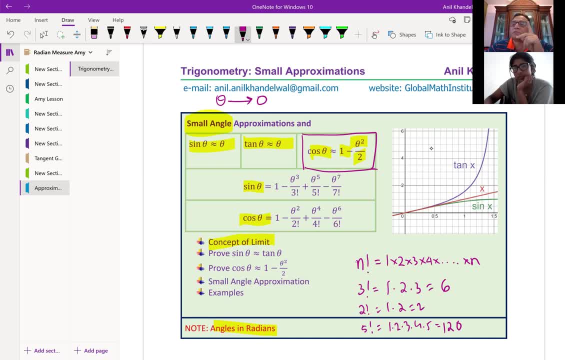 think like this: If you're looking at planets, right. If you're looking at planets very, very far away, like things like this, right. So you're looking at a very, very small angle. You get the idea. This angle is in minutes. 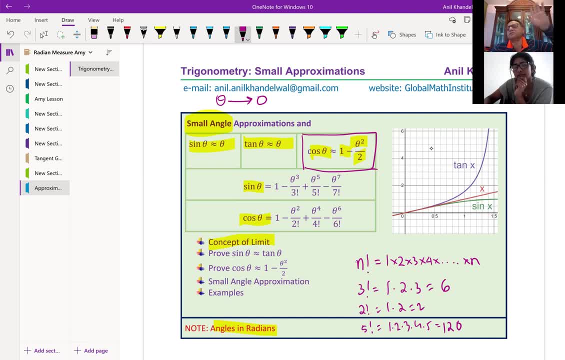 It's not even in degrees, Yeah, yeah, Because the distances are far, Right, Right, The distances are far. We're looking at very small angles. We could approximate sine theta to theta to do our calculation. Yeah, I see. 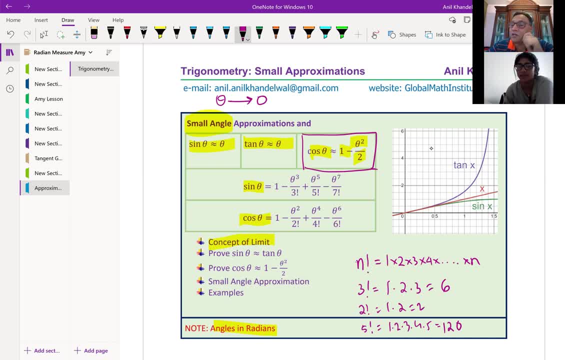 Sine theta to theta to do our calculation, You get the idea. Yeah, yeah, So the approximation is so accurate. Right, We can actually get fairly good results from those things. Is that clear to you? Yeah, Because when you hear approximation, 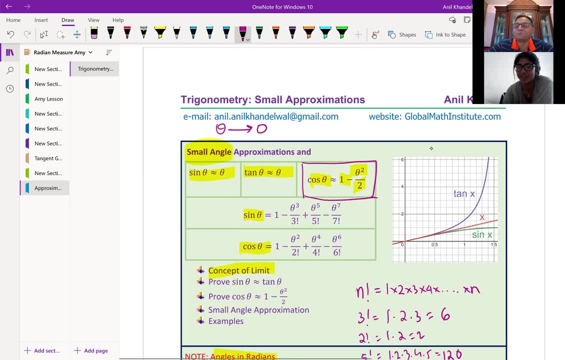 it seems like it's just like a wild educated guess, But it's actually quite accurate. Yeah, Quite accurate. Now, what I've done here is: we saw some graphs from your book. Well, fortunately I have very different ones. 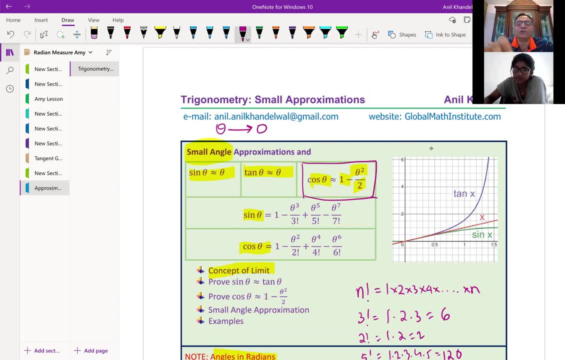 You know the approach is slightly different here. So what I've done here is I've shown you a graph of y equals to x. Do you see that y equals to x? graph right in the middle, Right The red one: Red one. 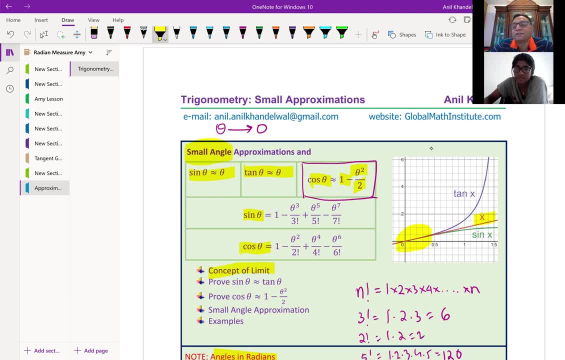 Now, if you look at this part, then tan theta and sine theta are both equal to x. Do you see that? Fairly equal to x. This is very enlarged, as you can see. This portion is like overlapping, Is it? 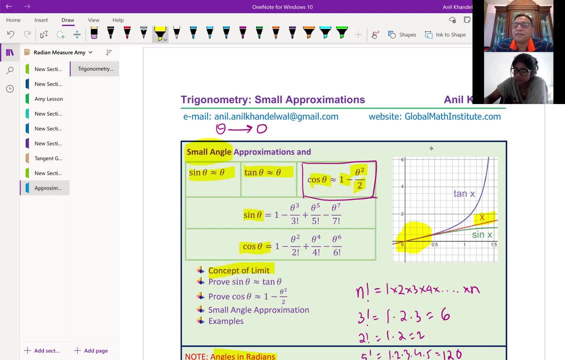 Yeah, yeah, But as we move along, you will notice that tan theta is is closer to x. that then, I mean, sine theta is closer to x than tan theta. right Second, you also realize: yeah, Does that mean that sine x? 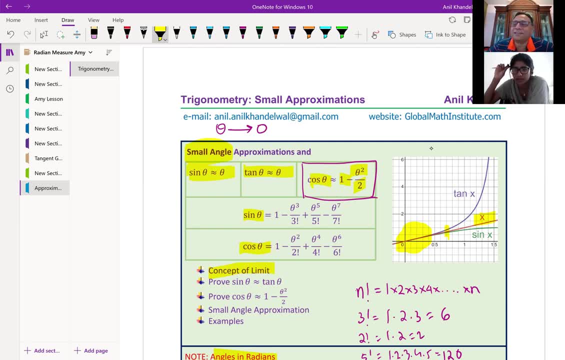 um, it's got a. the approximation is much more accurate. Yes, Yes, So the percentage error for sine x will be lower- Right Yeah- Than for tan x. Oh, I see, For the same value. let us say we pick up a value. 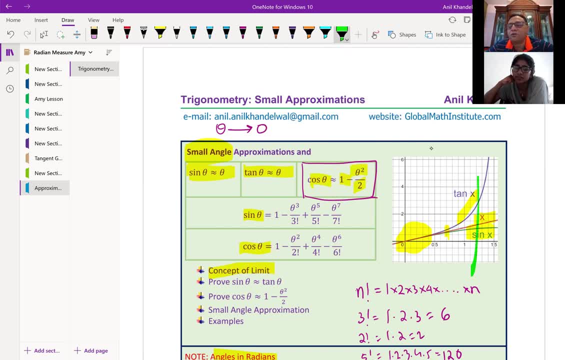 which is close enough. I'm, let's say radian value here right Around one, one degree, Let us say one degree right, One radian, One radian. If I pick up, then see for one radian. 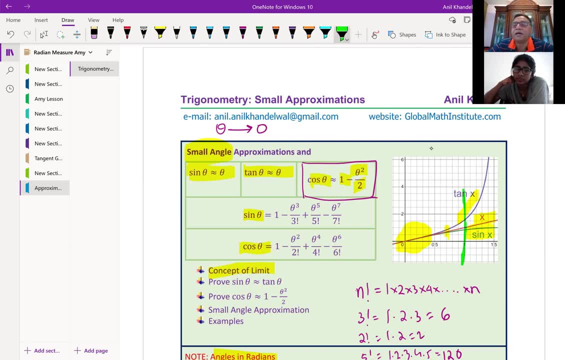 the percentage error for sign will be very small as compared to tan, because we are actually taking the x value. Is that clear to you? Yeah, Yeah. What do you also see is the tan value actual is higher than the x value and sine value is lower than the x value. 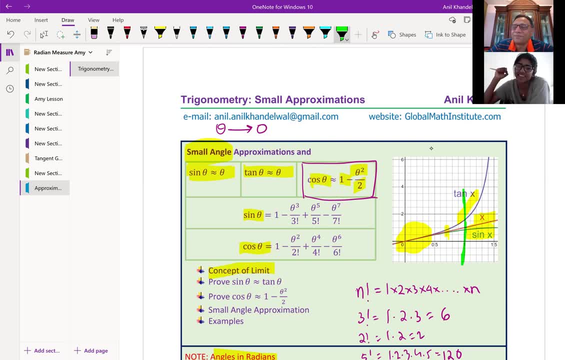 Yeah, So none of them are actually on the x value. That's why it's the approximation. Yeah, Okay, X is kind of mean somewhere in between, correct? Yeah? So all these things you can visualize from here Now in today's lesson. 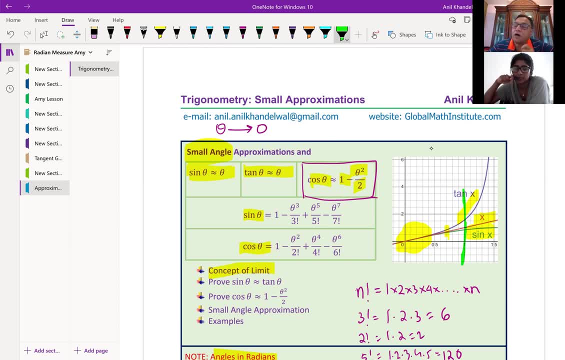 I'm only giving you an idea of what is a small value and how do we just calculate. in the next lesson we'll talk about percentage error in calculations and how much close can we go to the radian zero value? Is that okay, Yeah? 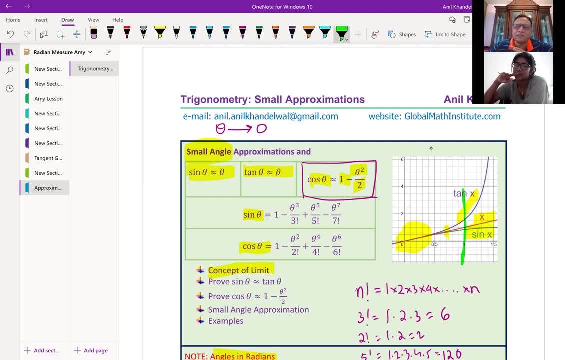 Just a percentage error in the next class. but let's try to understand the approximation itself. How accurate the approximation is and the type of results which we are getting is good to visualize is that tan theta value is higher than the approximated value, But sine theta actual value is lower than the approximated value. 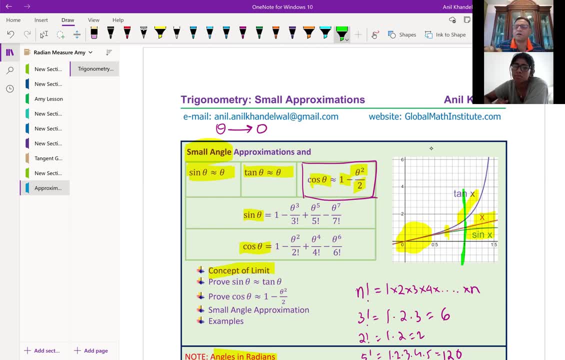 right, Because the x is right in the middle of almost is in between sine and tan. Is that clear to you? Yeah, So just a quick thing. So with the cos theta graph, are you not drawing it on there, because it's different? 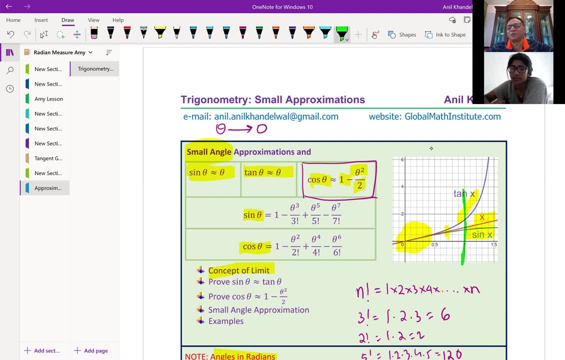 Yeah. Yeah, It's different. I'm not drawing on that. I should have drawn, Uh, but what I'm trying to do is like sinusoidal functions. When I discussed with you, I said: the sign is my main curve. 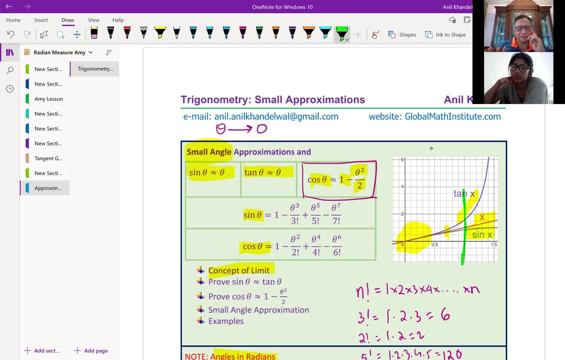 Sorry, Yeah, Yeah, Sign is a translated sign. Oh, sign is a translated sign, It's shifted Correct. Nine, So yeah. five by two, Yeah, So add zero cost. Theta is one, The value of cost data is one. 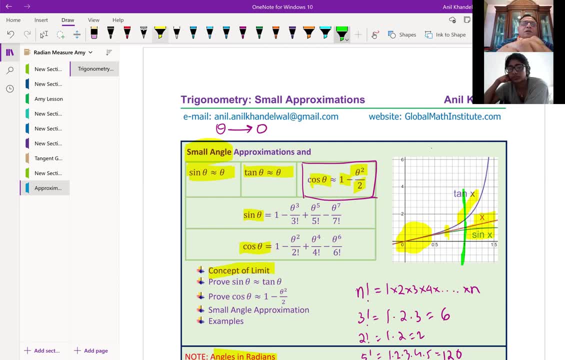 Correct, As you had seen in your book. this is a parable All right, Inverted Parable, All right. So if you draw this curve, I mean I, I need a different because for cost I I need at zero. 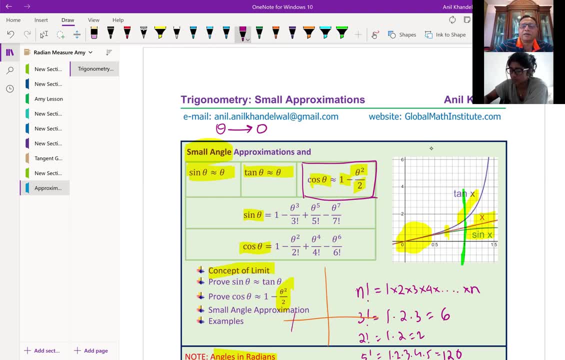 I mean, you get the idea for the cosine. the function will be kind of like this: Is that clear to you? Very different from 10.. Yeah, Yeah, So there's no. yeah, So it is a. it's a separate story altogether. 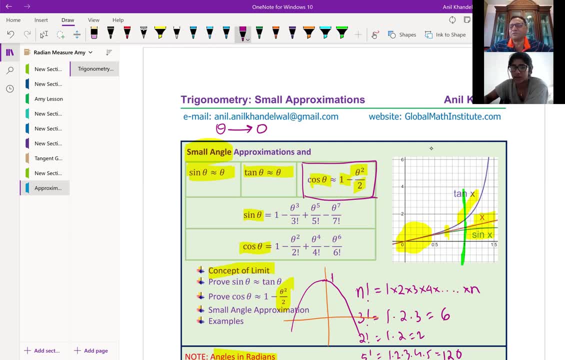 Right, So I thought I'll not mix and match. Okay, cool. Yeah, The way you drew the graph is quite clear to see um you know the difference between sine X and tan X and seeing the percentage error between them. 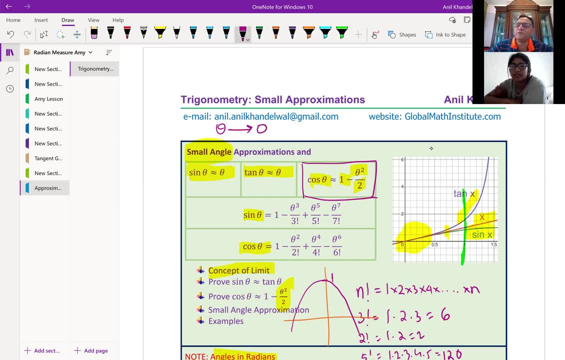 Yeah, So that's, that's what's appreciated. Sign and 10.. Correct, Yeah, And we. my interpretation to cause is I I say causes a function of site. Yeah, So the base. I will derive this formula of cause from sign. 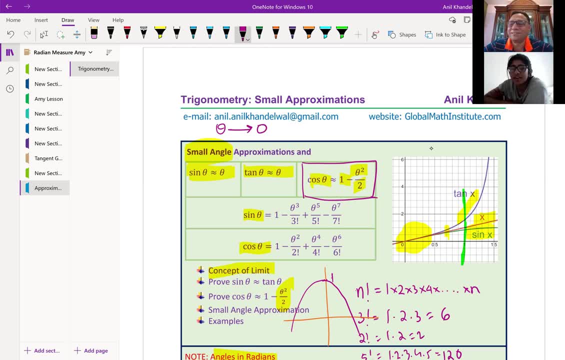 You can write right, I'll derive the cost from site. If I found a value with sign, let's just say: can I find the value, of course, just by shifting. Yes, Yes, Okay, You can definitely right. 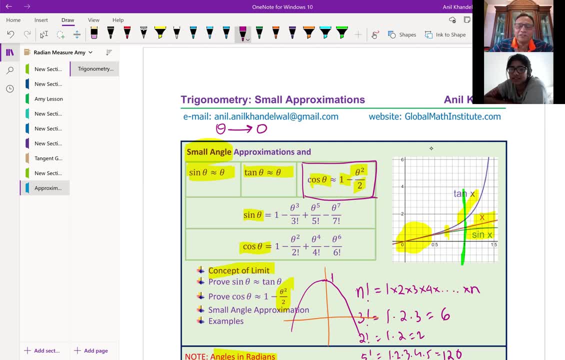 Yeah, Both are related. I'll show you how. I will show you how we. so okay, let's see. So first I'll talk about the concept of limits and then we will see how to prove that sign. Theta is approximately equal to theta. 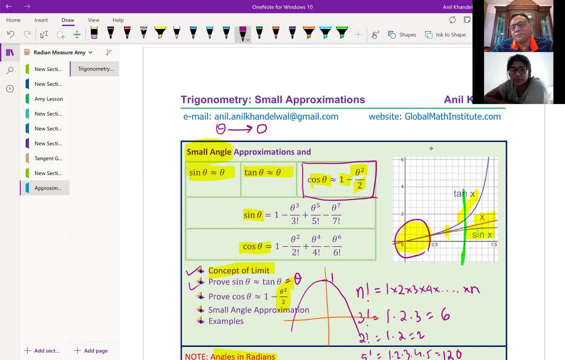 And both are equal to theta. right, You can see this portion right. Both of you can now appreciate that tan theta is actually higher than the value estimated. Sign data is lower than the value estimate. Perfect, Then we will prove that. 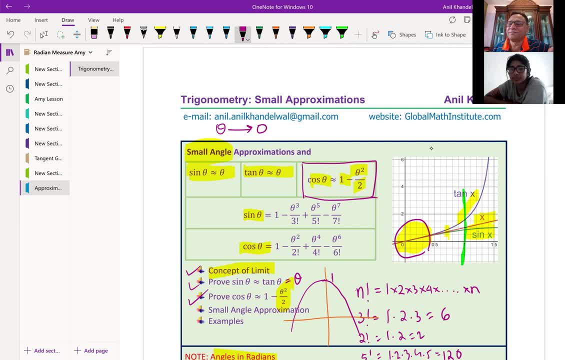 That cost theta is equal to one minus theta squared by two. We'll prove it Okay, So we'll. we'll start from here. We'll prove other things. right, We cannot start with so many assumptions. That is what I thought. 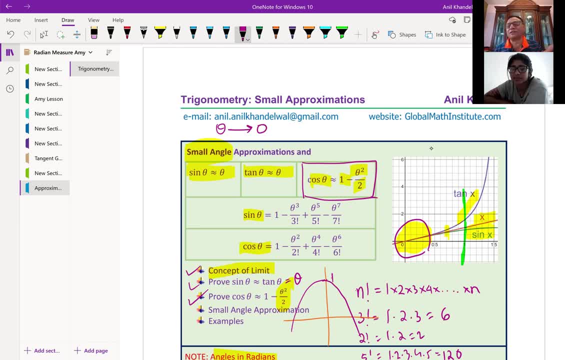 right, Right. If I give you, these are the formulas that now apply and get the result, There's no fun in it, right? How did you arrive at the formula is more important for me as a mathematician or a math student of grade 11 or 12 or 13,. 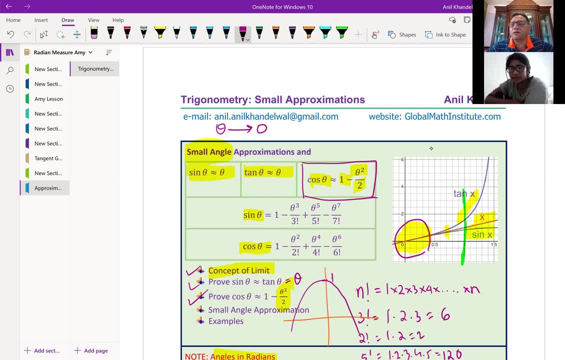 right Right, Right Right. We are not into like just this is the formula: Apply, Get the result. No, no, no, no, No. How did we get there? We have to understand. Then we'll take some examples. a small angle approximation examples. 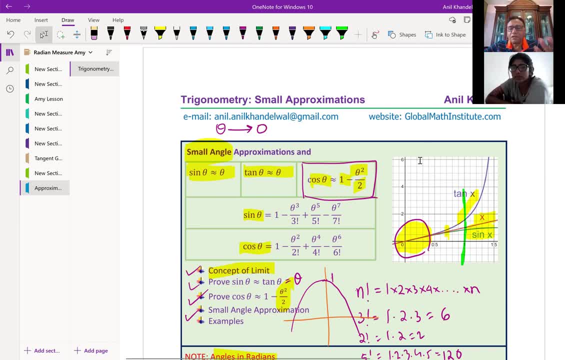 which are similar to your book, which I just saw. Right, Okay, Is this clear to you? Yeah, And this is something which you're good to know. So I'll say plus plus correct. Good to know, Not required. No. 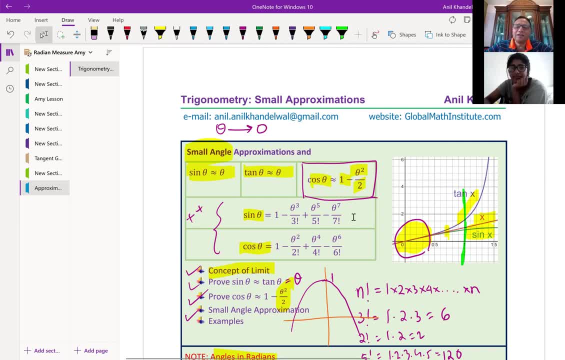 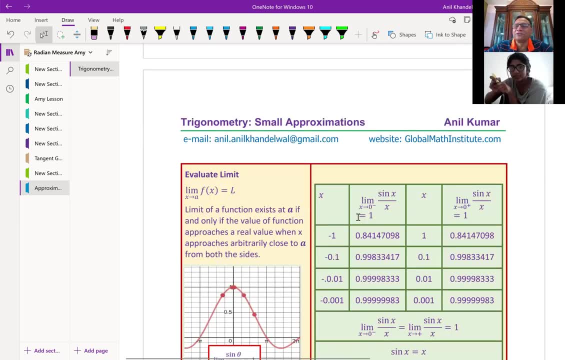 Okay, We'll need it after two, three lessons. Okay, Once we covered the binomial theorem. Okay, Yeah, Oh, I see. Yeah, Yeah, It's connected, Everything is connected. So I'm taking to calculus now. 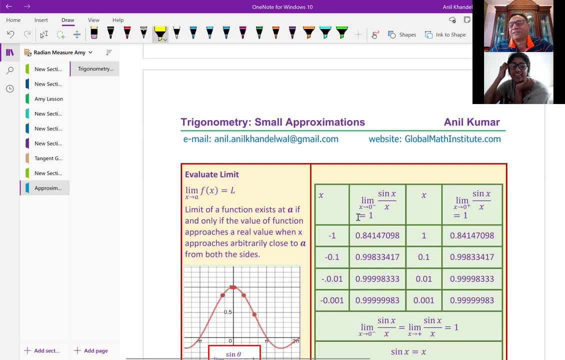 That's what I love Connections, Because trigonometry is such a vast it's a foundation for many higher level mathematics things. I can see it creeping up in every topic. Yeah, So we have a connection with binomial theorem series. 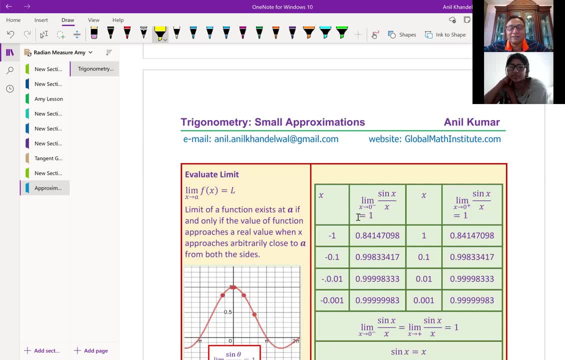 You see that series right Approximations: Yeah, This trigonometry is, with calculus, Correct, So it's very well connected. That's why we'll we'll understand it all, But in, you know, in steps, small steps. 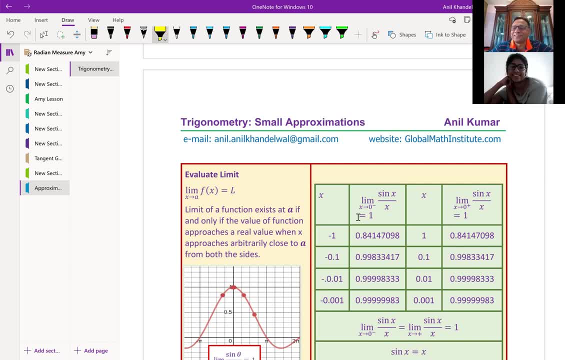 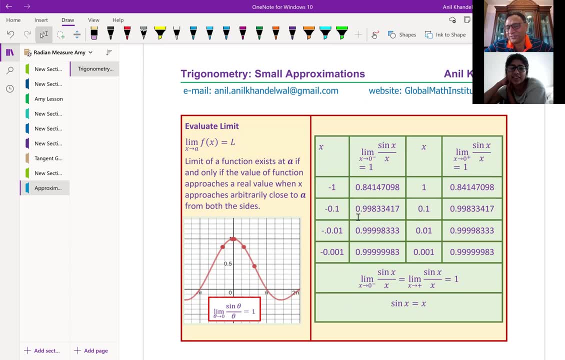 Steps. Yeah, So the graph which I have drawn is not the cosine graph. Let me tell you how this bell type thing looks like your cosine graph in the book. No, no, This is not your cosine graph. Okay, Not your cosine. 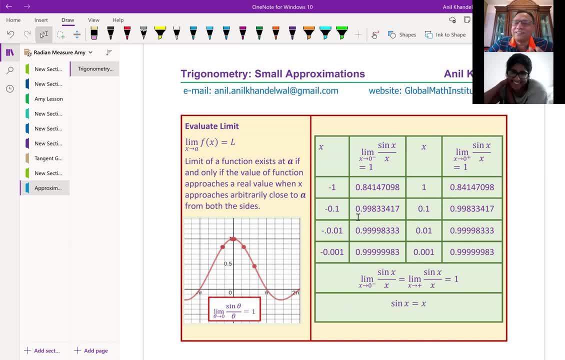 It is my, But it starts at one. Sine theta over theta function. Okay, So this is the graph of sine theta divided by sine theta. Okay, Okay So sine theta divided by theta, Is it okay? Yeah, Even though it starts at one. 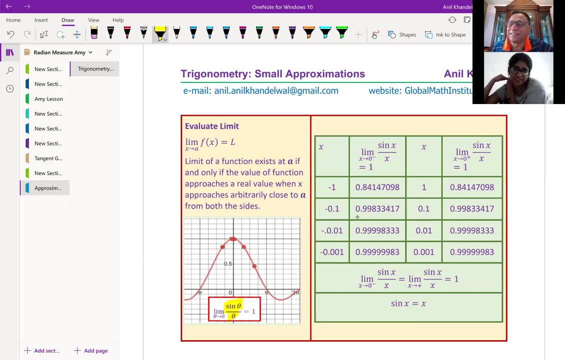 It looks like that. right, Yeah, Now it makes sense, because you said approximate value of sine theta: is theta, Correct? So if I divide sine theta by theta, I get one, Correct. Oh, So that is my one. That is my one. 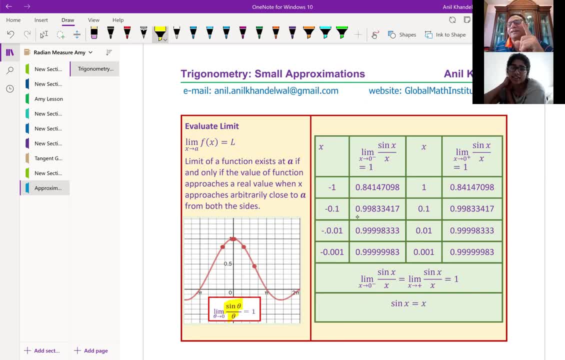 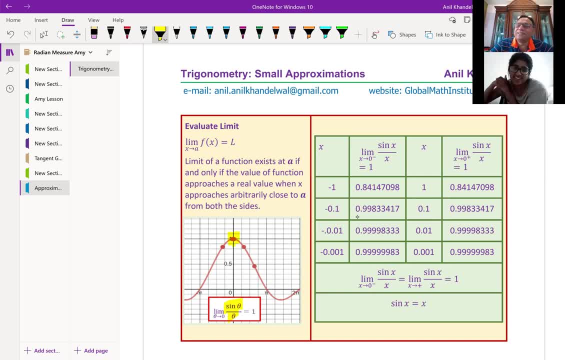 Yeah, approximately. Yeah, Yeah, Yeah, Yeah. So sine theta is Sine, theta equals theta, Sine theta equals theta, Is it? the angle is small. Is the angle is small, correct? So it is only one in this band. 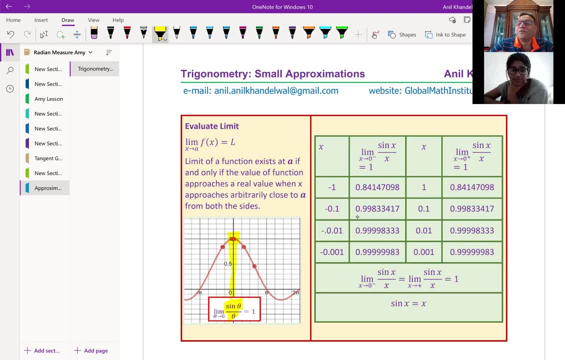 Do you see that? Oh no, we're off. What do you see? Otherwise, it is lesser value. Theta is there, So it makes sense. Yeah, We had a graph which was kind of like: this right, This was x right. 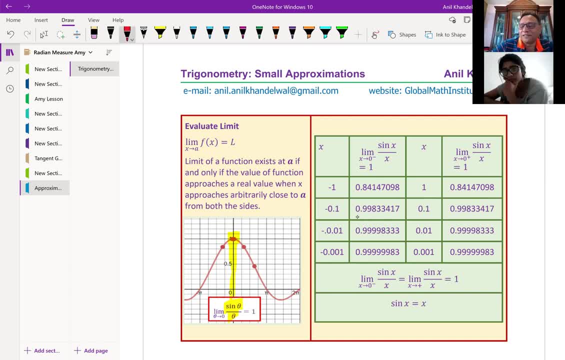 So let me again draw with the reading so that you understand. We'll keep following them. Great Yeah that. And I think that one was green, I don't know what. the white, the sine X, is green, Kind of like. you see that sine X, this is sine X. So it makes sense that that picture. 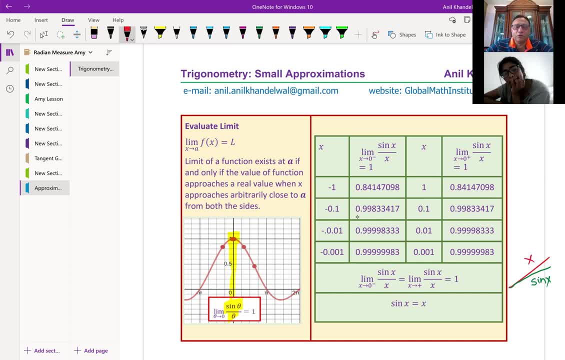 the first one. So you may call X or Theta if you want to. Theta and X: the same thing, Only very small. It is one, correct? Otherwise, sine X is lower and therefore you have a value. This ratio is lower. Do you see that lower ratio? Yeah, It could be anything, I mean. 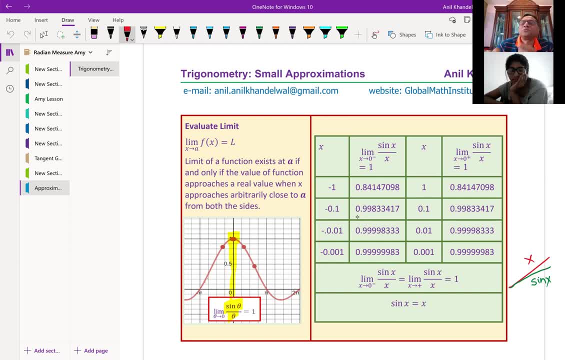 it's not. they are not equal. They are only equal in a very small band. This is what I'm trying to show. Is that clear to you? Very close or very small comes from this concept. It is only when we are approaching to zero. do you see? from left side and right side. 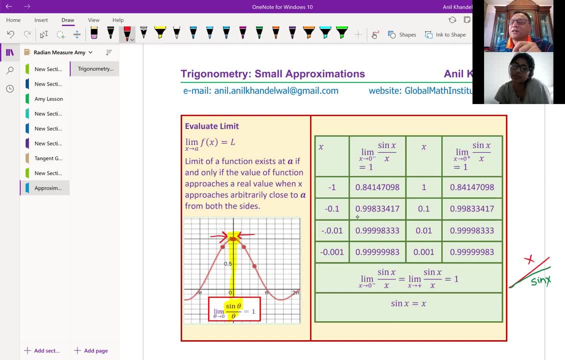 when you approach, then the value sine Theta over Theta approaches one, and then sine Theta equals to Theta, right. So that means now: sine Theta equals to Theta. I can cross multiply right When Theta is approaching zero. is that clear to you? Back again, I think now. 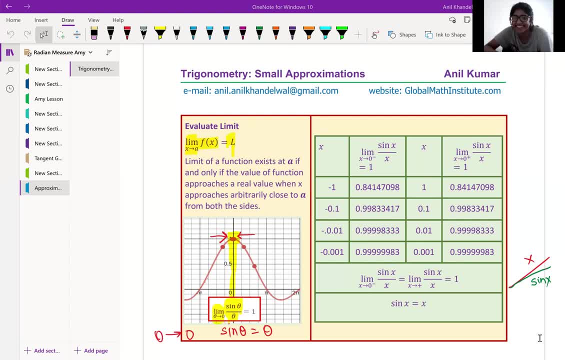 your wifi is fine, right? Yes, hopefully. Okay, You can see the screen? Yes, I can. So we were here. we're talking about ratio of sine Theta and Theta both measured, Theta being measured in radians. As you can see from the graph, when Theta is approaching, 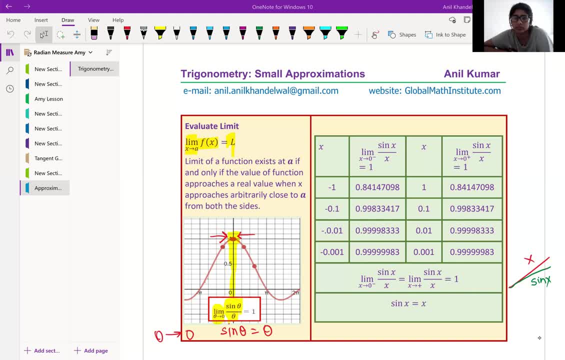 zero from both sides, left or right. in that case, sine Theta over Theta is one correct, Yeah, So that basically means that sine Theta is equals to Theta When Theta approaches the value zero, correct, Right. That is what we. 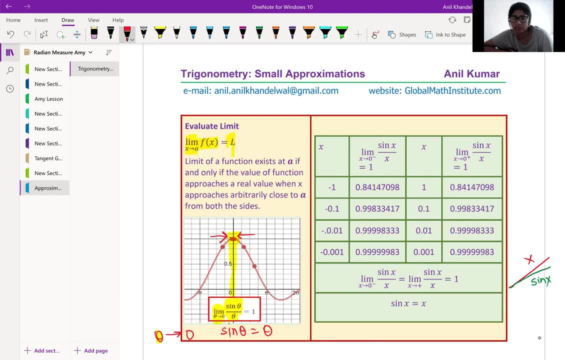 have come to now How close you can see from here that only a small band was very, very close, which I've highlighted in. Yes, yellow is the portion where it is approximated sine theta and theta same, But if theta is slightly 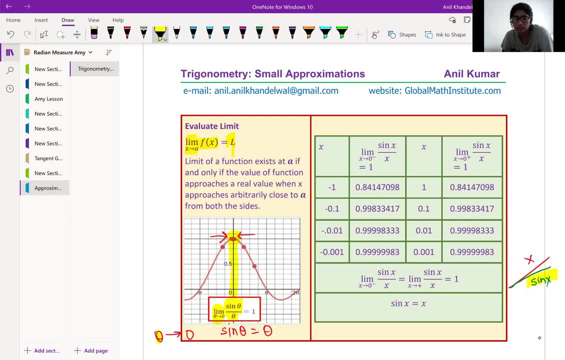 more. then you can see that sine theta value is much lower. right, As we had seen in the very first graph, y equals to x is slightly above. y equals to sine x, correct, When we are talking about small angles Now in limits, what we do is that approaching means. let us say we want to. 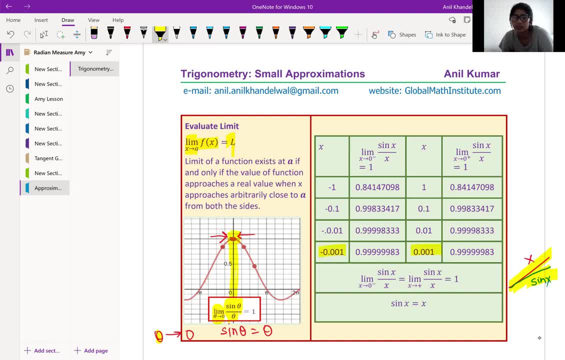 approach: a value zero. zero from left side and zero from the right side. It really means that minus one to minus 0.1, minus 0.01,, minus 0.001 means getting close from the left side, correct, Oh, okay, Yeah, closer to zero Moving from the right side. you can start with one. 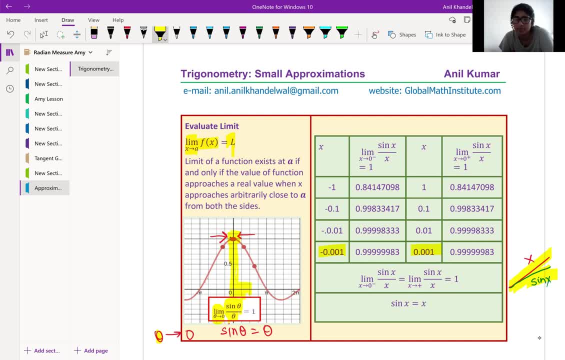 for example, and then move towards the closer to zero means: test the value of sine theta at 0.1,. test the value of sine theta at 0.1. And 0.001, what do you get correct? Yeah, So if you calculate this value sine x over x, 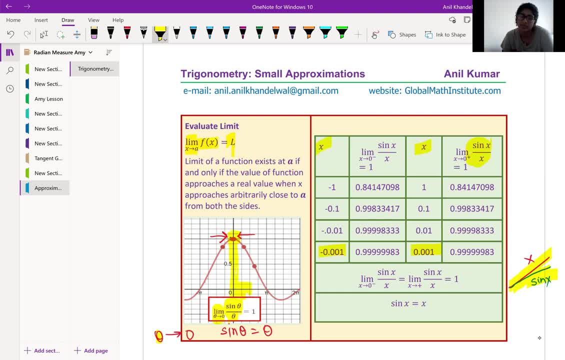 for these values of x given in the table, then the column shown here is approaching from the left side. The column shown here is approaching from the right side. Clearly, 0.9999 means they are approaching one correct From both the sides. Yeah. 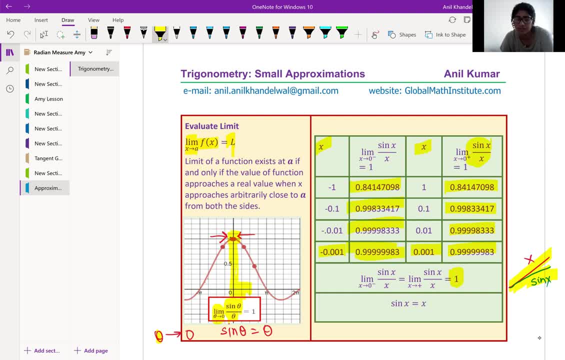 Perfect. So I cannot divide by zero. When I have sine x over x and x approaching zero, it cannot be zero, correct? I cannot divide by zero. We're talking about approaching means very close to zero. You get that part right. Yes, sine zero is also zero, It is true, But we cannot. 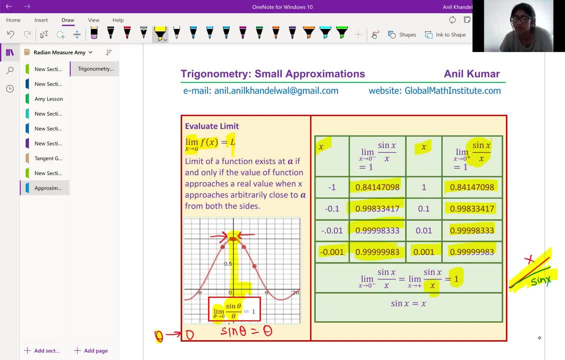 write sine x by x at zero, because the denominator cannot be zero, Perfect. So we use this nomenclature approaching zero very, very close. So at this stage, sine x is equal to x, and that was your approximation. You have understood how. 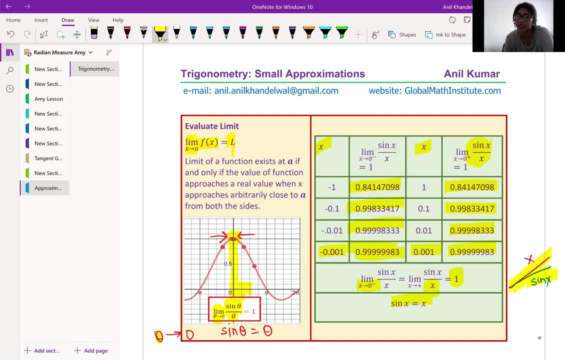 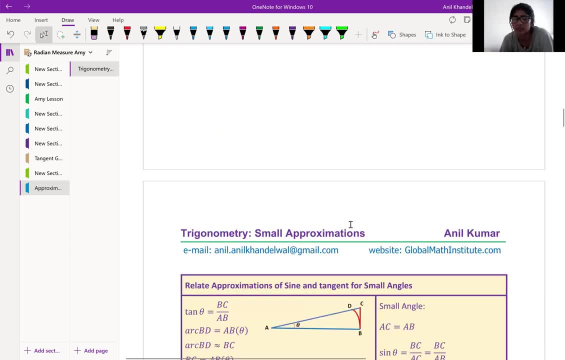 and why do we have this approximation correct? Yeah, really clear. Absolutely, you're right. Now let's see about the tan x. We know tan x will be slightly more than x from the graph. we just saw it. But now let us see how exactly we can, you know, derive it. 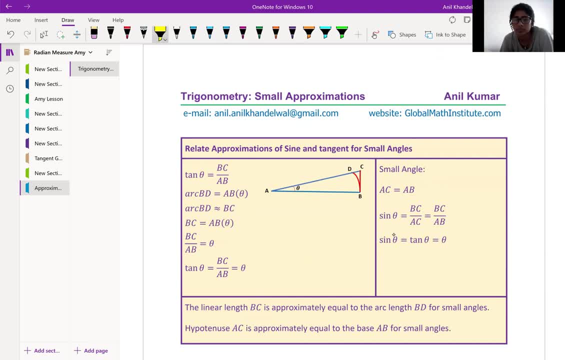 So here what I've done is that I've taken a segment a b. This is my segment a b, Now made a right triangle a, b, c. So in this particular case I have a right triangle, angle 90 degrees. 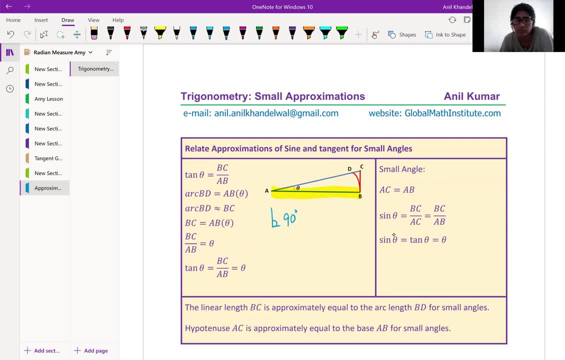 at b, right. So angle b is 90 degrees. So my triangle a, b, c is the right angle triangle, Clear, Yeah. So in that right angle triangle what is tan theta equals two. If this theta is a very small angle, then tan theta is the ratio of 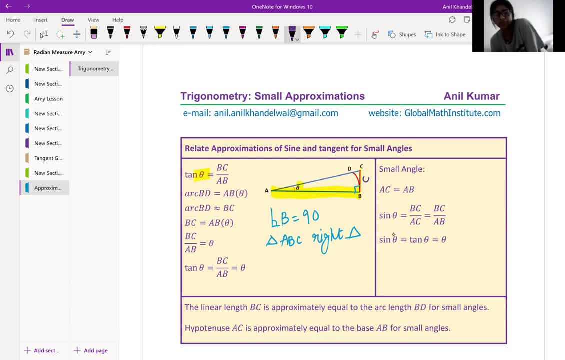 opposite side to adjacent. correct To adjacent, yeah, And clearly it is b c over a b, correct. Now, if the angle is very small, then this r, which I've shown in red color: b d, d, b, yeah, b d. 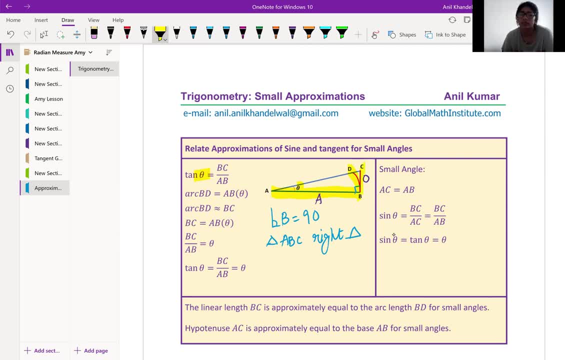 It will be same as b c. correct, It will be same as b c, because if the angle is very small, then this angle is very small. So if the angle is very small, then this angle is very small. They will overlap, correct. Oh, okay, Yeah. 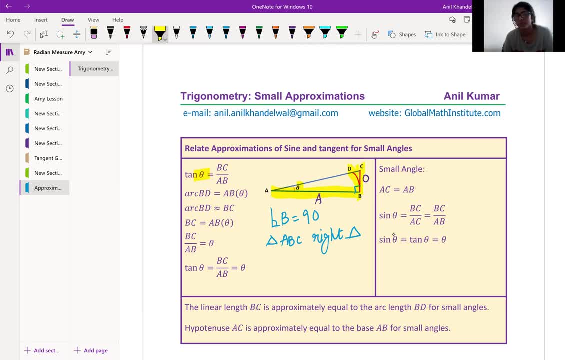 What is r? You just learned? r is r, length is r Is r times theta. r here becomes a, b correct. So a b times theta is the length r length b d correct? Oh, So that means this r length b d is same as b c. So I've written that this r length b d 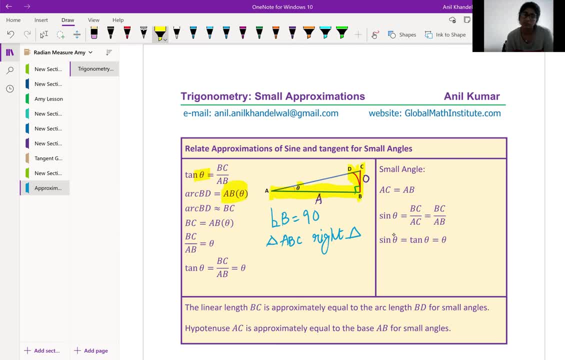 which is a b theta, because the radius for this r is a to b distance. correct, Yeah, So a b theta is basically equal to a. b theta is basically equal to the opposite side: b, c. 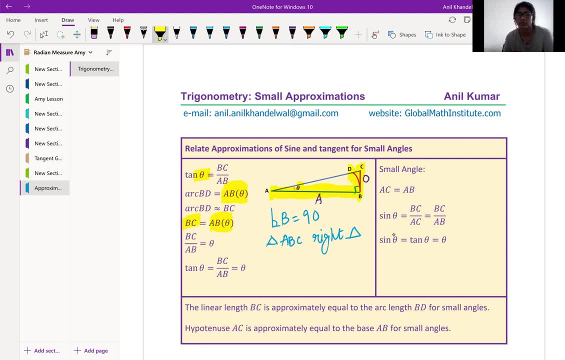 correct, Yeah, Now what is the ratio b c by a b? Just divide b c by a b, you get theta. So b c by a b is theta. That really means that tan theta, which is b c over a b, 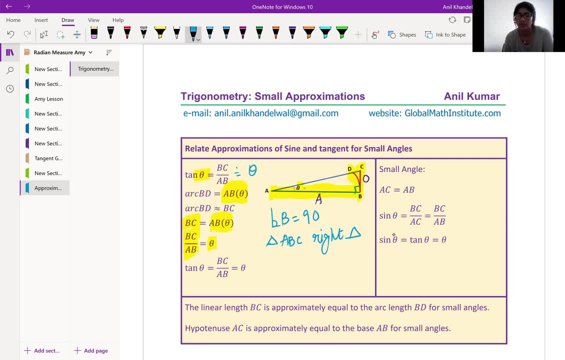 is approximately equal to theta. when angle theta is very small. Do you see that? Oh, yeah, yeah, Clear. That's why I actually did, actually before I even knew this when I was doing on my calculator, because it's in radians. now when I do tan over like 0.26, my value is also like 0.26 something. 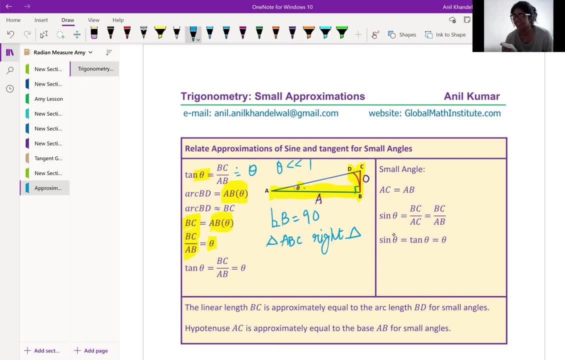 Yeah, And I'm like: why is that happening? But I thought it was just coincidence, I should have questioned it. Now it makes sense. Oh, okay, Clear, Yeah, And it didn't happen with cos, only sine and tan. 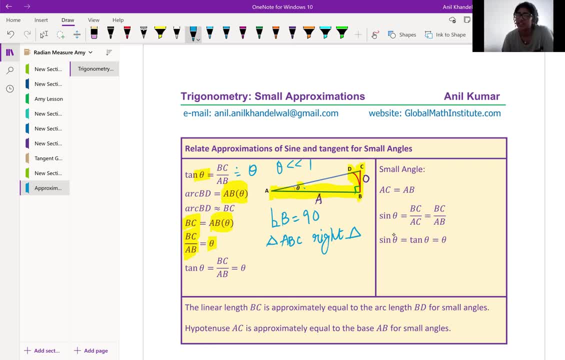 With cos also, it will happen. You didn't notice, but it will happen. Oh, it does. Yes, Oh right, So you clearly see that tan theta is also equal to Theta. Yeah, We earlier derived: sine theta equals to theta. Now we are saying tan theta equals to theta. 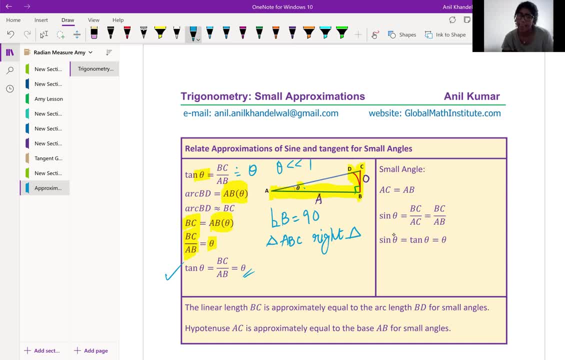 Both are same right, Almost same. You know, tan theta is slightly more than theta sine theta is slightly less than that Lower, But they are almost same. Now we could also approximate this longer length ac to ad correct. 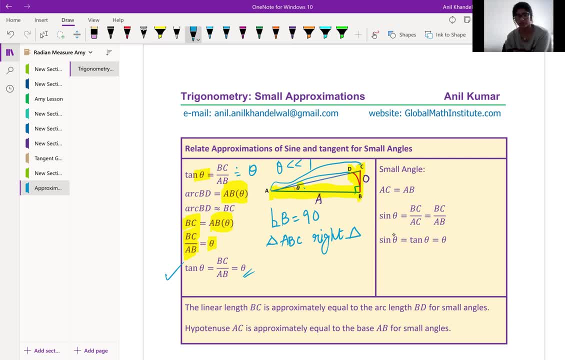 Because the theta is very small As we approximated the arc to bc. Now, if I approximate that, that is the hypotenuse we are talking about, Do you see that? So a positive over hypotenuse, which is the sine theta right, Bc over ac, which is sine theta. Now if I'm saying a to c is same. 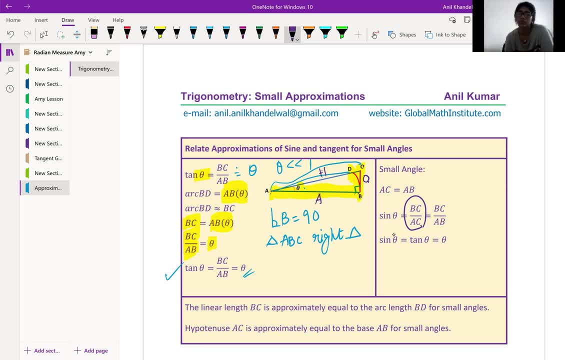 as a to d right, Which is same as a to b right. Yeah, So it is the same as tan theta. Yeah, Bc by ab correct Makes sense. yeah, And therefore sine theta and tan theta, both approximate to theta. 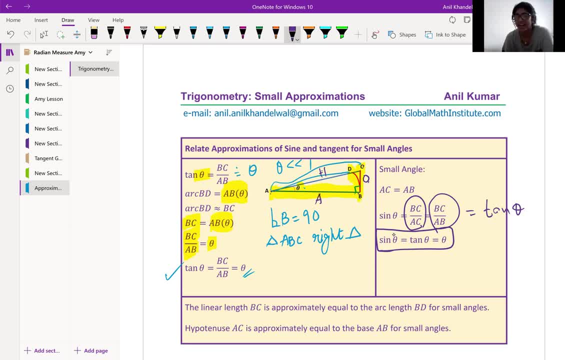 That's clear. It's good to see how it was derived. yeah, So it is from this particular side that when the angle is very small, the arc length is actually equals to the linear length between those two points. Oh, got it, Yeah, yeah. 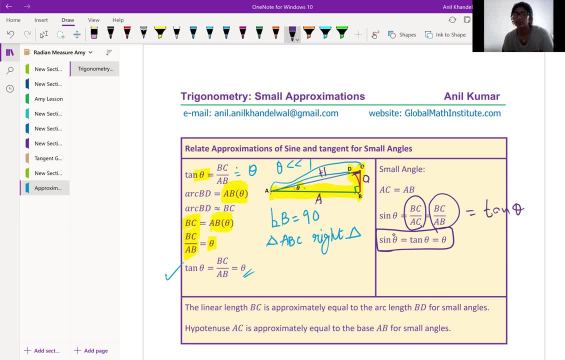 And then that these two points are supposed to be same. Yeah, So that's fine Hypotenuse. it doesn't matter, right? Whether you take this distance or that distance. So tan theta and sine theta are the same, right. 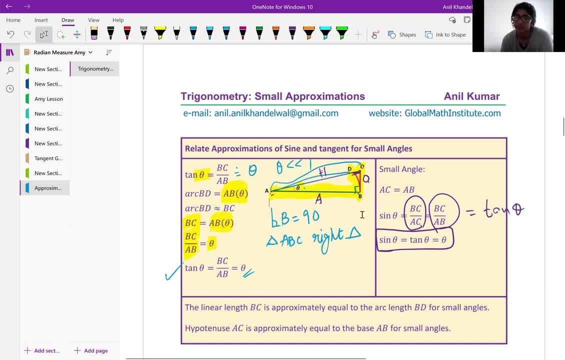 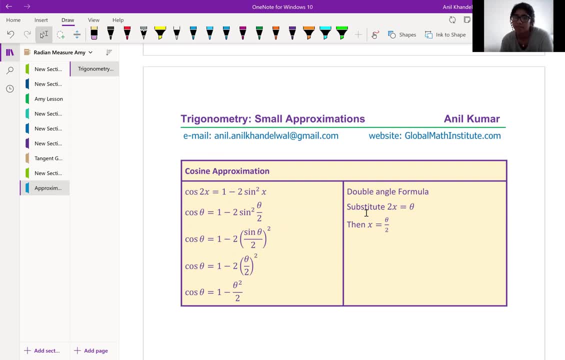 Right. So that is how we derive it. Now let us get back to cosine theta and understand how cosine theta's formula is derived, which is one minus theta squared by two, because it's very different from tan and sine results correct. 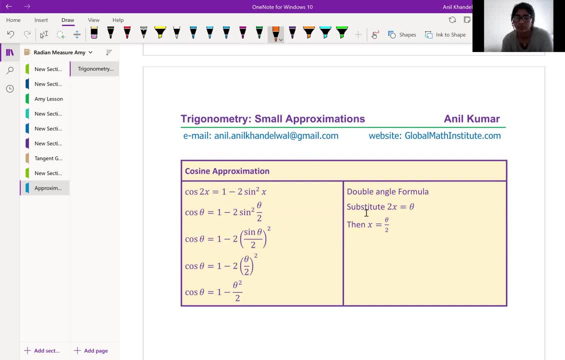 Yeah, yeah. So let me take you to the trigonometry of compound angles. in that we learned some formulas right. So we had the formula of cos A plus B, which is cos A sine B, cos A cos B minus. 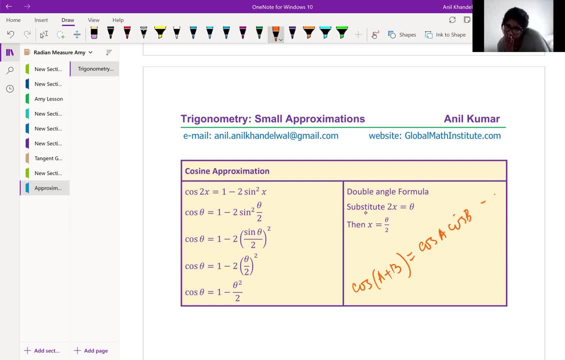 sorry, cos A, cos B, minus sine A, sine B. And from there, if I put A and B as same, if I put A as equal to B, Yeah, So I get cos of 2A, if I write B equal to A, So we get what We get cos I'm writing. 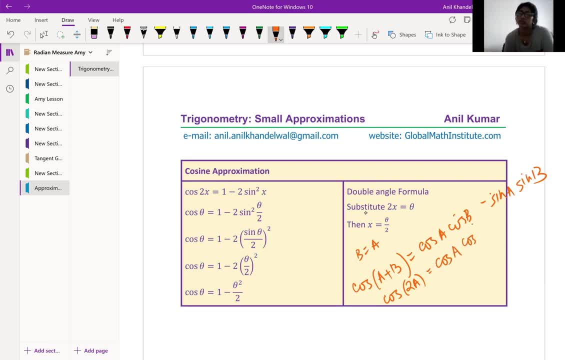 B as A. so it gives cos A times, cos A minus sine A, times sine A. correct, Yeah, That gives you cos squared A minus sine squared. Now you could write cos squared A as one minus sine squared A. Yeah, And you have here sine squared A. So you get the formula one minus two sine squared. 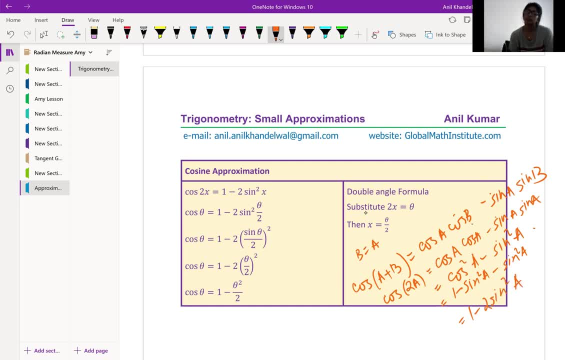 A. This is a standard formula which you also might remember. So we say: cos 2A is equals to one minus two sine squared A. So that is where I'm beginning from. cos 2X is one minus two sine squared X. okay. 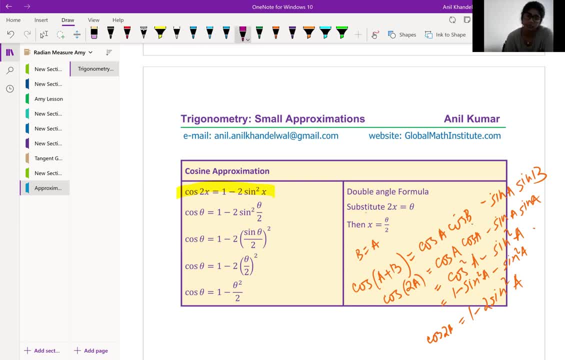 Yeah, yeah. Now if I substitute 2X as equal to theta, that means 1 minus two sine squared A. So if I substitute 2X as equal to theta, that means X is equal to theta by two, right, If? 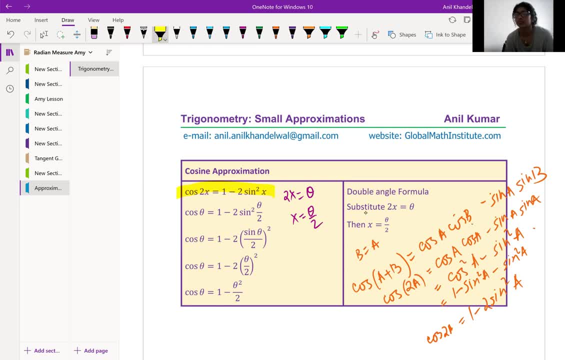 I do this substitution, I get cos theta. I'm substituting instead of 2X theta is equal to one minus two sine squared instead of X theta by two. You see that, Yeah, yeah, We just derived which I sine squared theta by two. I could write like this to be more: 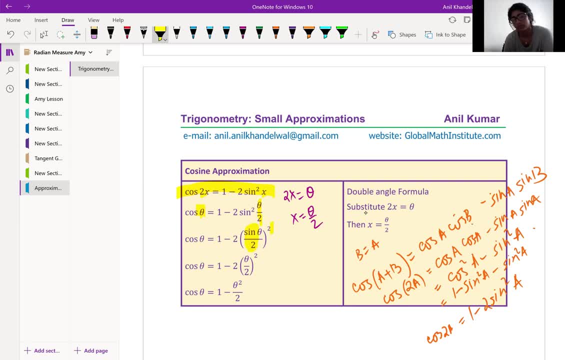 clear. Yeah, We have just said that sine theta is what Theta, right, Yeah, So Theta is very, very small. Let me write like this: as compared to one, We're talking about radians. Sine theta, In that case, sine theta is theta. So we get one minus two theta by two whole squared. 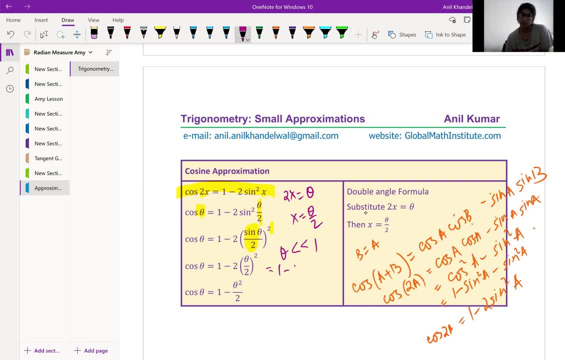 which is what Theta squared by four, right? You could write this as one minus two, theta squared by four, correct, Yeah? And then you cancel two and four, you get theta squared by two, which is the formula for cos theta. Is that clear to you? 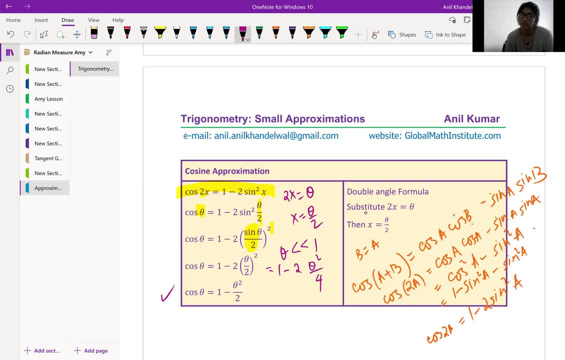 Right. So that is why I'm not giving you the graph for the cos theta, but I'm just deriving the result from what we just derived. Yeah, Makes sense, Makes sense, Yeah. So this is your cosine approximation. Now you've understood all this, Let's take some. 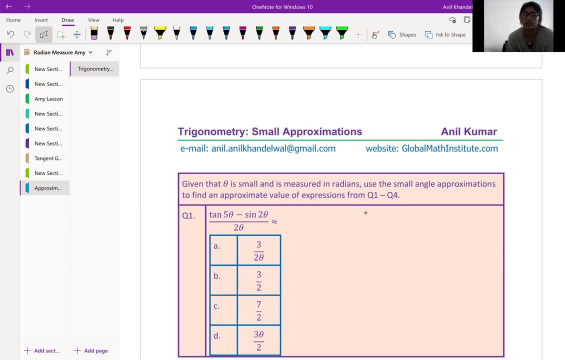 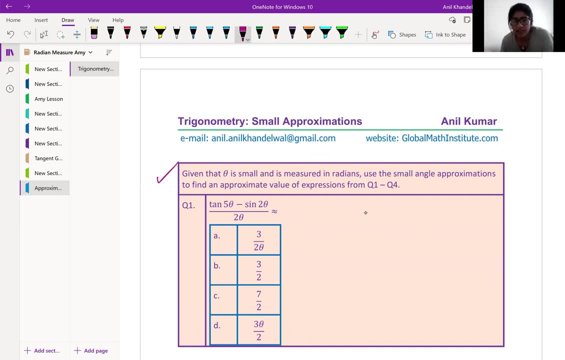 examples. So what I did was I took multiple choice questions. you know it'll be easier for me to explain, So can you please read the first question? Yeah, So given that theta is small and is measured in radians, use a small angle approximations. 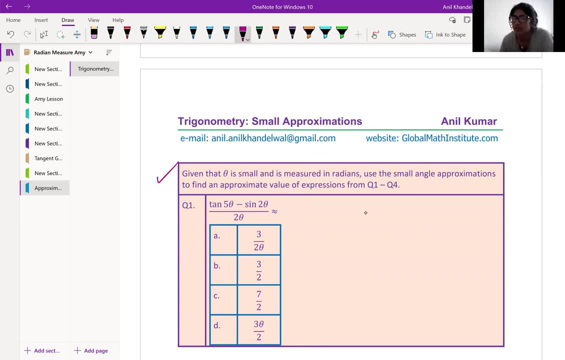 to find an approximate value. Yeah, So you can find an approximate value of expressions from question one to four, Correct, So we have four questions. First one: tan phi. theta minus sine, two theta over two theta should be approximated to which value Let's calculate. Tell me Tan phi. 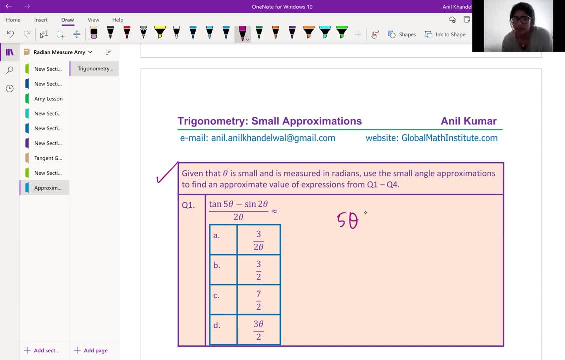 theta is Five theta right. Five. theta minus two. theta Minus two theta correct. Divide by two theta correct Three. theta over two theta is three over two B. So simple. Do you see that approximation chapter? Yeah. 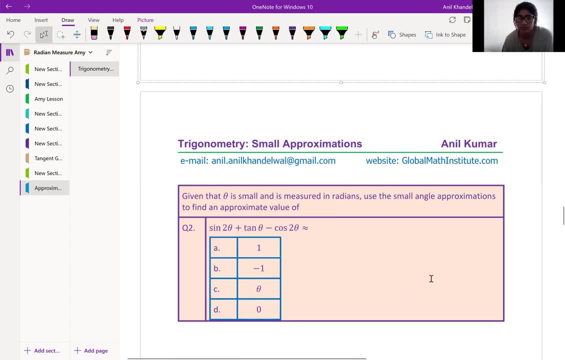 Very simple. Now question number two, but it's important to understand this one. Our thing is same, right. We'll just repeat it: Two theta plus theta minus one minus two theta squared over two, Correct, Yeah, So we need to simplify. 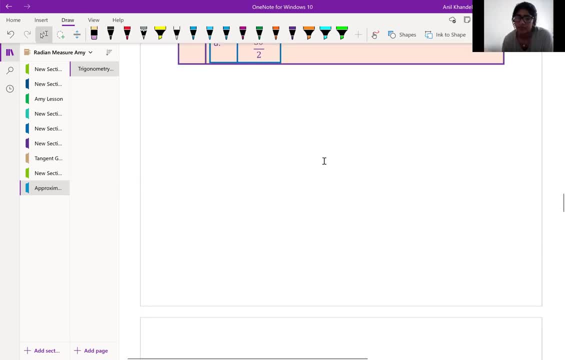 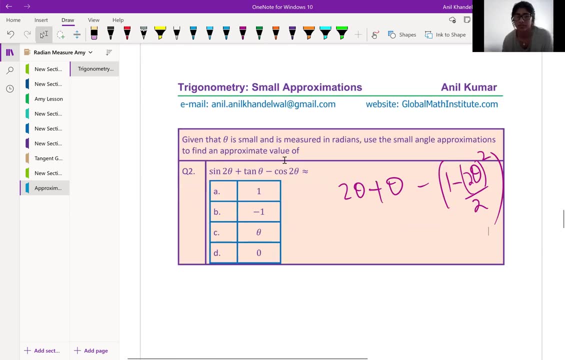 Right, So you have to remember this, right. So make a note of the formulas, because this cos theta formula is plucked from the formula. Okay, Then what do you do? So we keep the theta square over two, one minus theta square over two, correct? so we substitute this value. 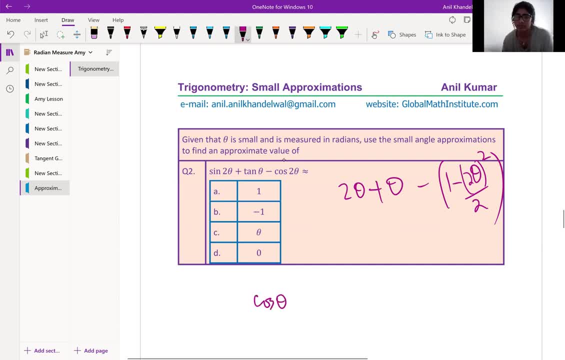 which is: let me write down here, right, cos theta equals to one minus theta square by two, right? so in this case theta is actually two theta. that's why we are putting theta square by, is it okay? so it is three theta minus. when you open this bracket, it is minus one plus two theta square. 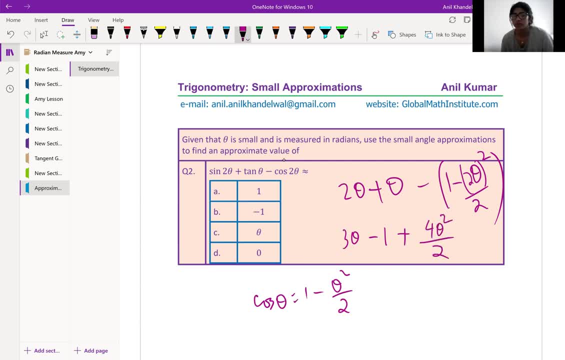 means four theta square, correct. yeah, over two. so that's two theta squared. so so what do you get? um, so two. so actually it was a product. i'm sorry, this was a product not multiplied. this is product. two weeks, this was not plus. it is a typing error, oh sorry. okay, um, so that would be. 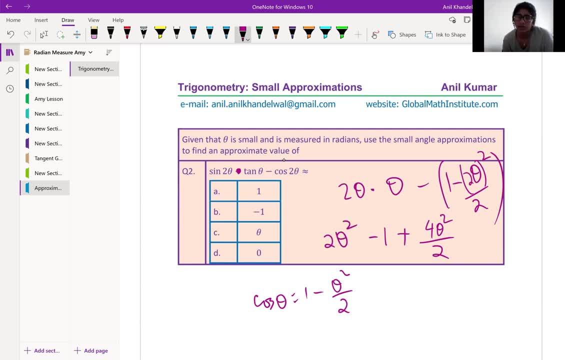 two theta square, sorry, sorry, two theta square. is that clear to you? yeah, oh, so it's minus no. so two theta squared add two theta squared is four theta squared. oh, but is that a subtraction for a whole? okay, so the answer is minus one. yeah, yeah, minus one. there was a typing error. it is product of. 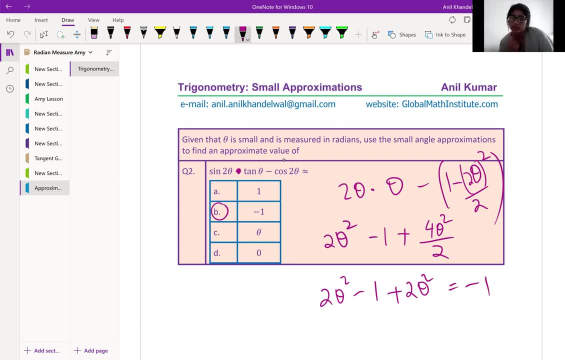 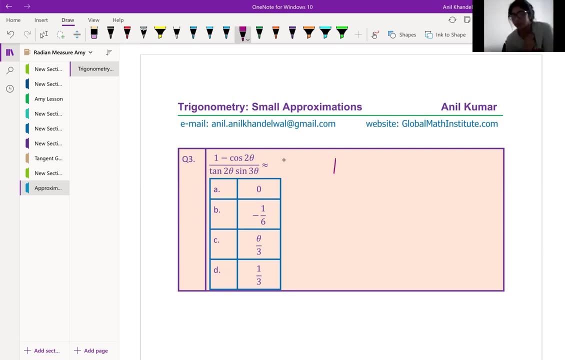 sine two theta and tan theta minus cos of two theta is bought correct. all right, yeah, typing. so that is what you do and you get minus one. there was a typing error. minus one as your result. clear, yeah, yeah, yeah, this one third. so one minus um, then in brackets: 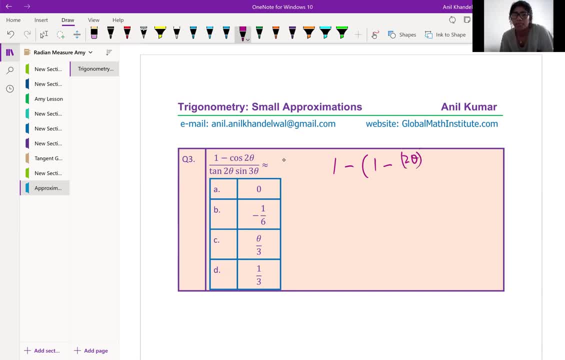 one minus two theta squared over two, divided by two theta times three theta, so six. so one minus one is zero, right. that becomes plus four theta squared by two. right divided by two. theta squared over six. theta squared, which is a third d clear, oh yeah, so you just need to know your formulas. yeah, that is all. so once the formula. 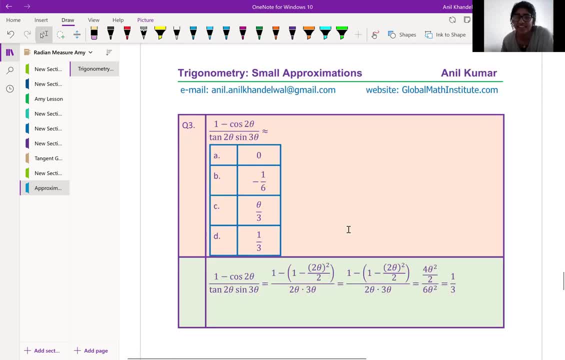 is given to you the exercise. there's nothing in it. you get the idea, oh yeah, but it's not nice to know how it? yeah, because when you taught me how it derived, and all the graphs and everything, obviously because this is quite so far like kind of easy topic, like you said, you just need to know. 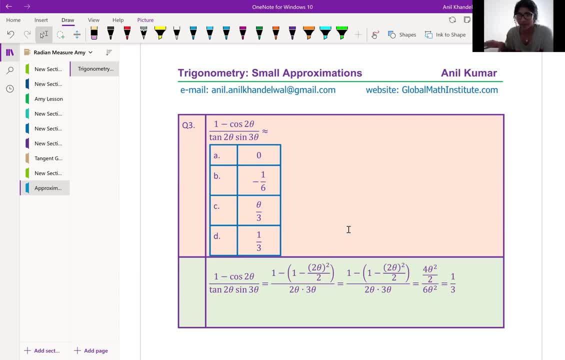 your formulas. but when it comes to the exam, because everything comes in one go, it's so easy to forget this. so knowing where it comes from it's really handy. yeah, and remember in the exam: this will not be an independent question. before this question, they are going to ask many 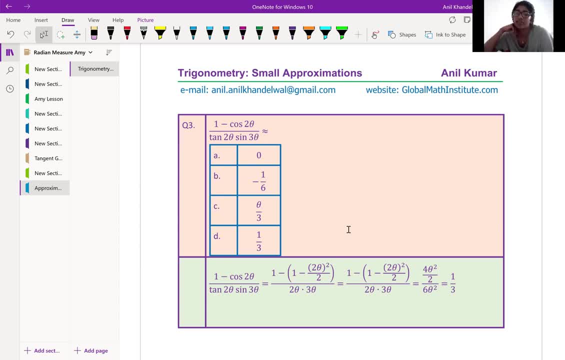 where you need to understand the concept. let's say, first find the arc length, they may start from there, and then what is your percentage error? right, yeah, but the part which you wanted to know is this, which, directly from the formula, is so simple. well, in this case, i've just 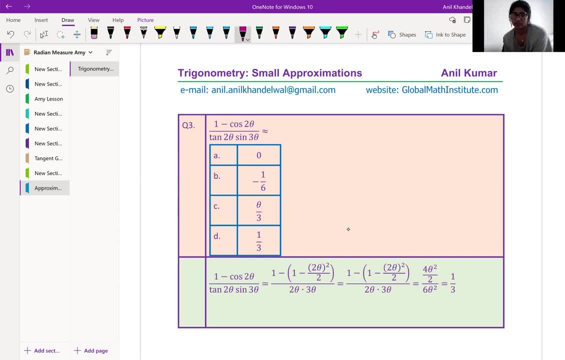 shown you the calculations: one minus cos two theta over tan two theta sine three theta really means one minus one minus two theta, whole square divided by two, divided by two theta times three theta, as we did, and you get the result one over three, and that is the right answer, clear. 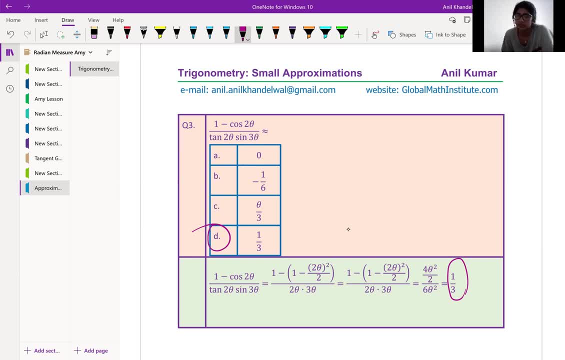 simpler, but that is how you have to do it. remember that when we are approximately approximating, then sine theta is approximately equal to theta. tan theta is approximately equal to. you can write: theta and cos theta is approximately equal to one minus theta square by two. now last question. 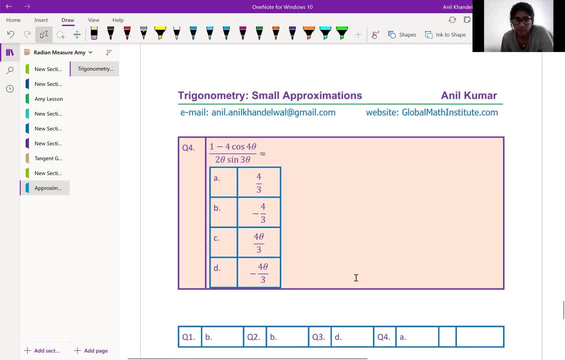 where we are just four of them. okay, so last question here is: one minus four cos four theta divided by this. can you quickly do it? so: one minus four times one minus four theta squared over two over two theta times three theta. so we need to simplify um one minus so that's gonna be 16 theta squared times four. 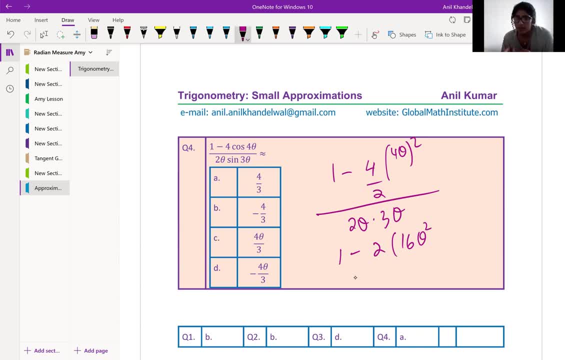 um 64 theta squared. so, yeah, i think you're times. sorry, there was one minus here, also sorry, sorry. sorry, there was one minus, right? oh, yeah, yeah, right, right, so that one, one and one will cancel. so we get plus correct. yeah, i'm sorry, okay, so two times six theta squared, correct? so one and one cancel, we get two times. 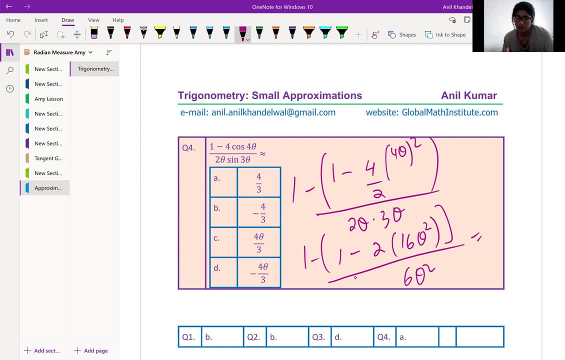 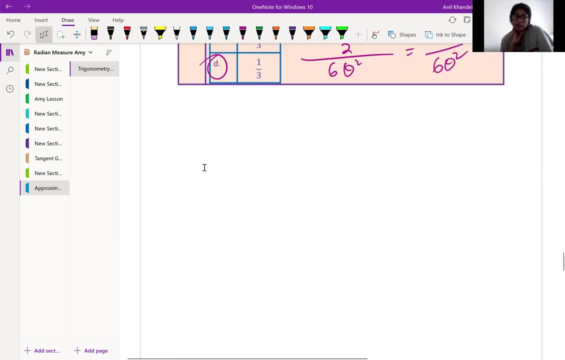 this three you could divide right. so 32 divided by six um four thirds. yeah, is that clear to you? yeah, yeah, so that is how you have to do this unit. so we'll end here, uh, for now, but i hope you understood the concept. the whole idea here was to understand the starting point. 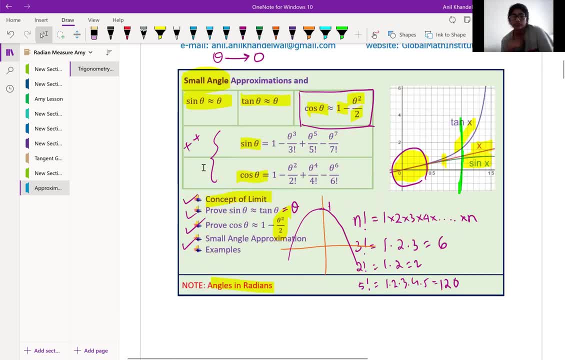 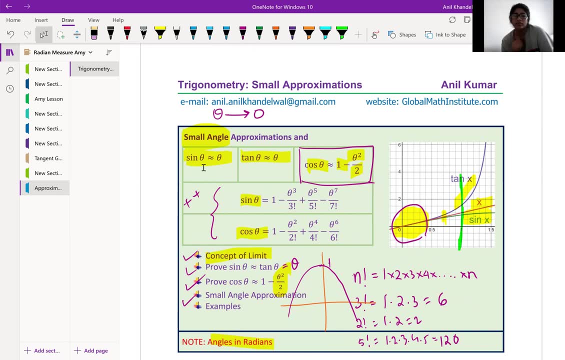 itself. that is small angle approximation. how do we get there? so sine theta is equals to theta when theta is very small. you could see that if i actually calculate the value of sine theta over theta. so the whole idea is that the value of sine theta over theta equals one equals to one when theta 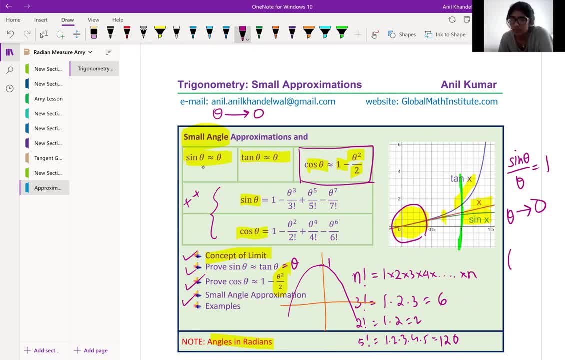 approaches zero. zero, that is what we say when theta is very, very small as compared to one. this is the base right. so we calculated, literally substituting the values of theta from, let's say, minus 0.001, correct, and then also check the 0.001 plus side, both sides, both sides, yeah, and we approached to a. 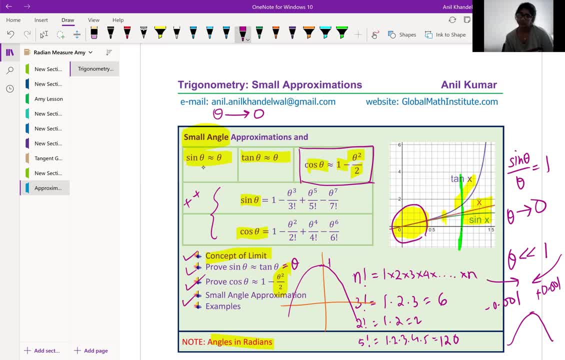 value which was very close to one, and you saw that graph which looked like this. so, only at very close to zero, it was one, right. so that is the foundation. and then for the tan theta, we had that art correct, so we had that r which gave you the concept. this is the arc, right. so and and if i kind, 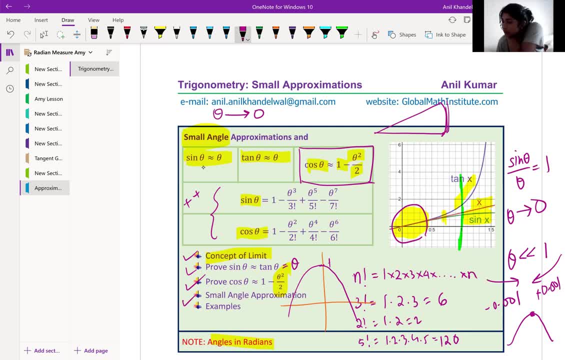 of extend it a bit further. i mean, you understand. so it make a right triangle, then the arc length is as good as the length of these opposite side and therefore tan theta. it becomes equal to theta and even the hypotenuse approaches the actual length which is base right and therefore approaches. 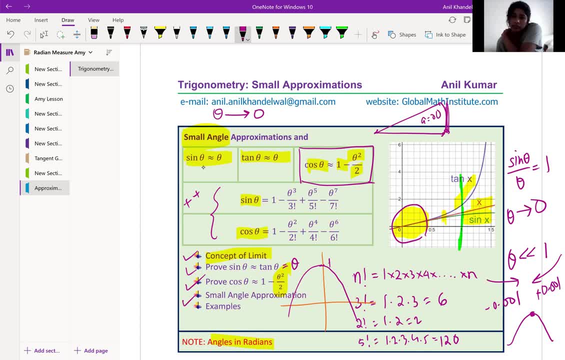 is theta and you know arc length a equals to r theta. so that is the, the formula which we use to find these results. is that clear to you? and using the cos 2 theta formula, we derived what this is when theta is very small, correct? so that is how we did all these. 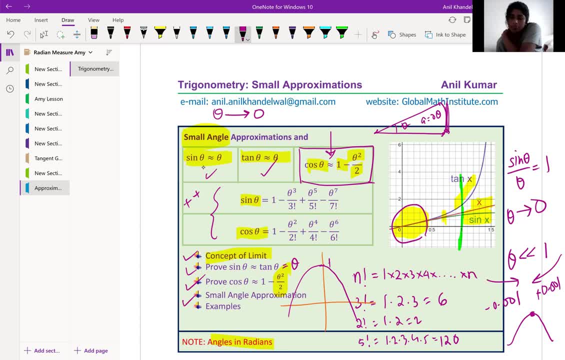 you know approximations and got the result. applying these results to the questions is not very difficult. you can substitute and get to this. in the next lesson we'll talk about the percentage errors and we'll also see which are good angles. up to what angles should we really? 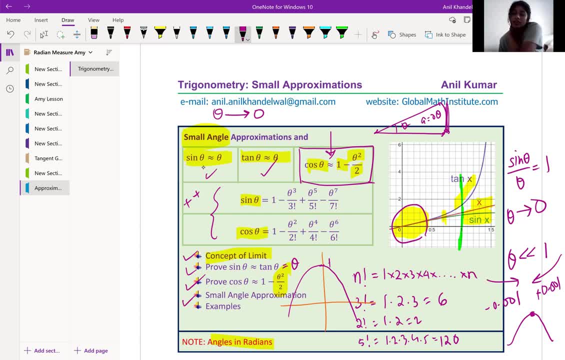 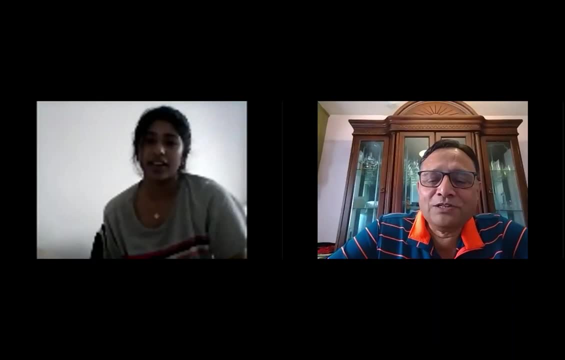 apply this approximation and if we want to work within tolerance of, let's say, one percent, right? yeah, in that case, what could be the maximum value of angle? theta, right? oh, i see that is the type of question which we'll look into next. is that clear to you? yeah, sounds really good. so, yeah, i think i. 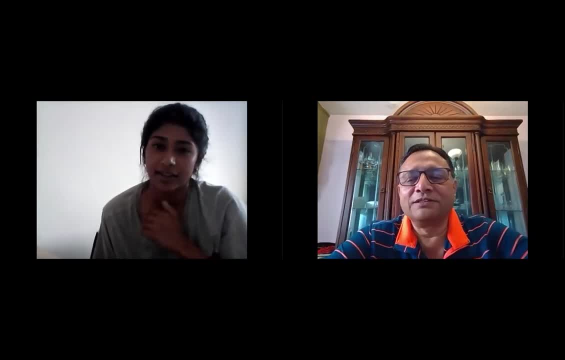 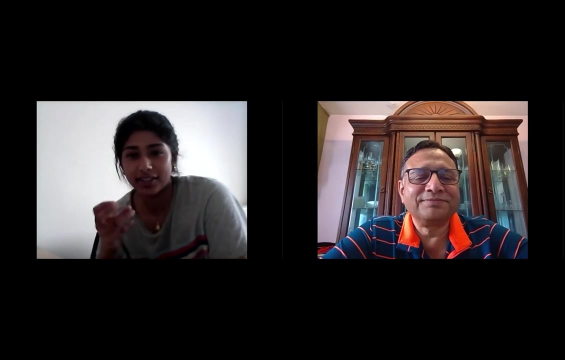 really understood this concept. so i'm going to end the class here, but i'd like you to kind of conclude what you have learned and summarize our learnings today. so yeah, like i saw when i shared in my book, it kind of just started off with the formulas and gave a couple graphs. but, like you, 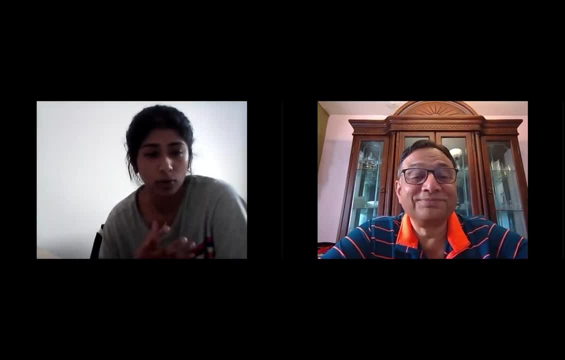 said. so i think it was kind of starting at the end and i kind of read it a bit more, but there was nothing else in my book. it was just that and that's where it starts. so i think, giving all that background on how those three formulas are derived and especially how 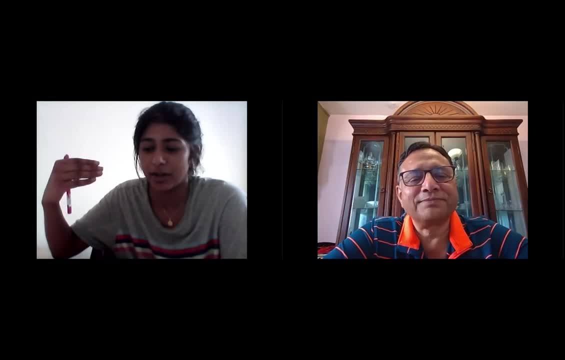 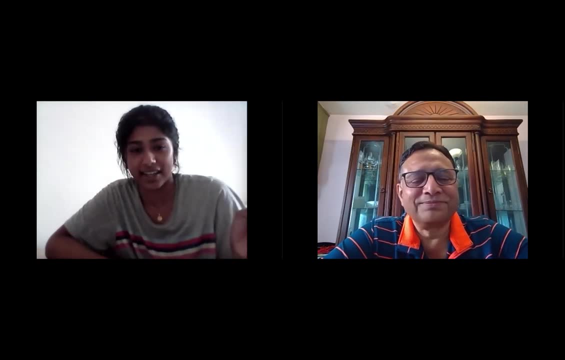 the graphs. look, because that was really clear to see. and um using that sine x. so, like you said, when subbing in those values, i don't think you can get it any more clearer than that. when you start at, like we said, um 0.01, just getting smaller from both sides, and seeing that eventually you're. 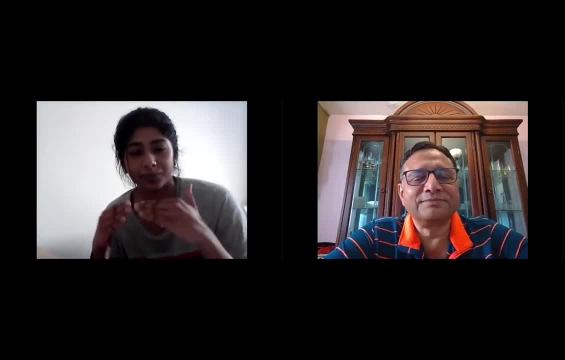 getting 0.99. it is one that's as close as you can get it, so therefore, using that when, when it approaches zero, sine x over x has to equal one. and so that's where, when you cross, multiply sine x over x has to equal one, and so that's where when you cross multiply sine x over x has to equal. 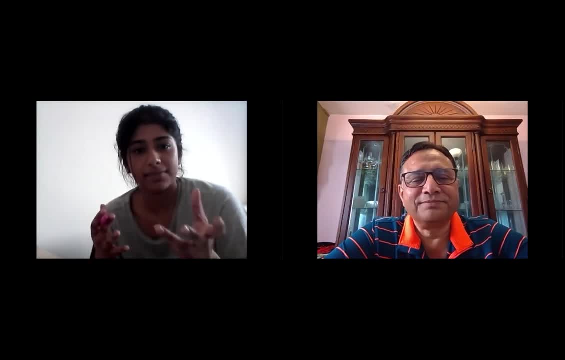 sine theta equals theta or vice versa. so we saw the same thing with the tan graph and then cos i'm glad you didn't graph it on the same one because it is a different graph, but seeing how it was derived is really was really clear. um, and just making like b equals a and working with that i